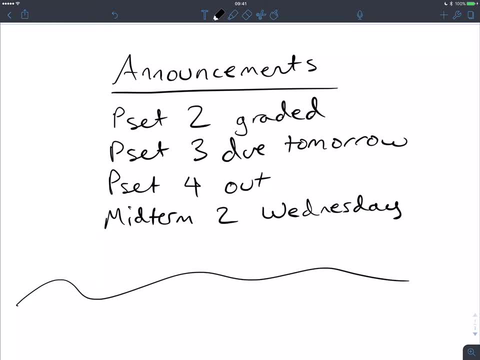 Pset 3 is due tomorrow, so any questions about Pset 3?. Pset 3 is due tomorrow, so any questions about Pset 3?. One variable Pset 3 is due tomorrow, so any questions about Pset 3?. 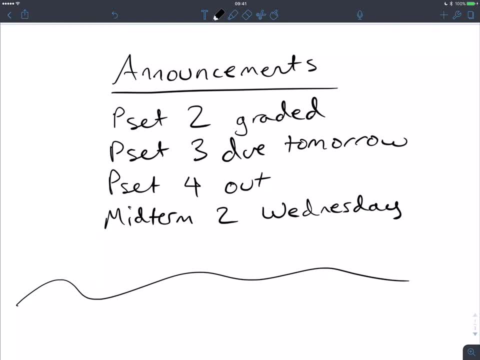 One variable. Pset 3 is due tomorrow, so any questions about Pset 3?? One variable: Yep. so you match any particular character that pushes on a symbol with any other transition that pops the exact same symbol. So first you have to massage the PDA so every single transition either pushes and doesn't. 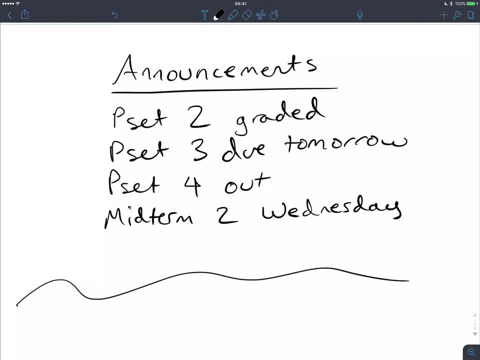 pop or pops but doesn't push, and therefore you are guaranteed to match correctly, But every push with a matching clock. Other questions about pset3?? Yeah, So problem number three, which is about shuffle of alphabets, I'm trying to make up a proof. 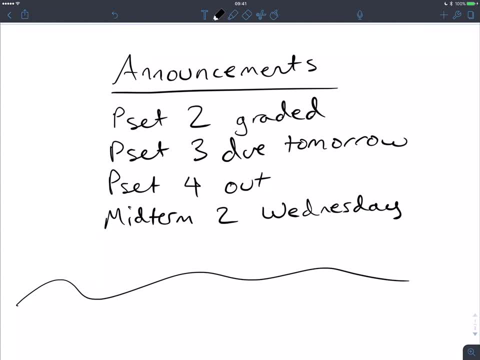 I'm not sure what we're supposed to do with that. It doesn't say anything about that. Pick your favorite language over any alphabet, Over any alphabet. Yep, As long as it's some language or some over any alphabet, Okay, Any alphabet. 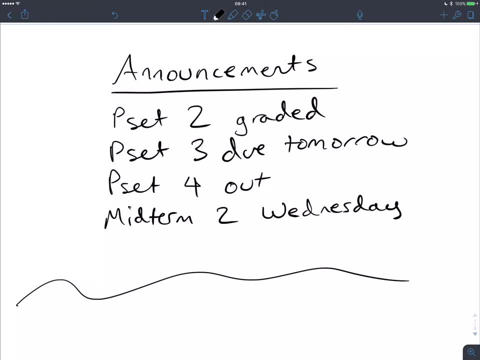 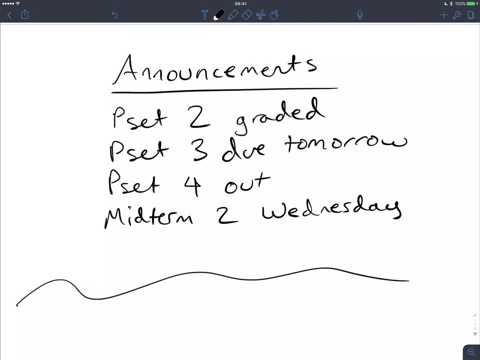 seen or any non-context-free language we've already seen. just cite it. Okay, Like if it happens to be 0 at the end, 1 at the end, 2 at the end, just say: we proved that this is not context-free in class. 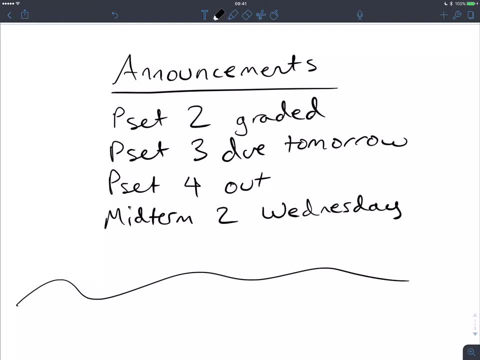 Okay, Okay, Thank you, Yep. Other questions about pset3? No, Okay, Okay, Okay. So I did get a couple questions about question 1.. So for the conversion from PDA to CFG, limit to at most 50 rules for each of the three. 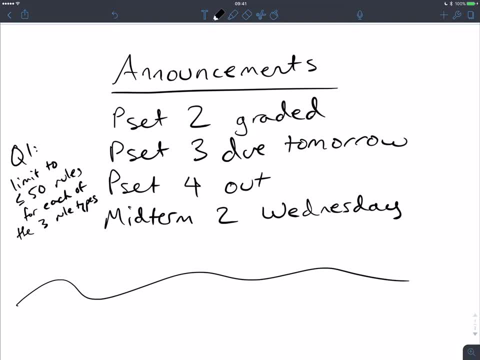 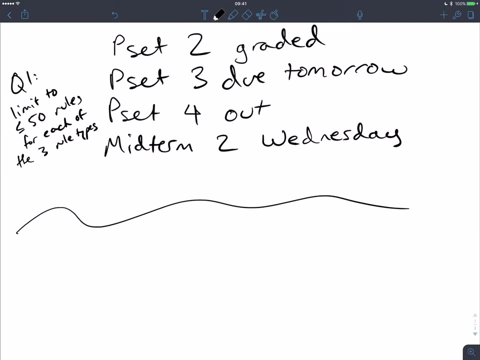 rule types. Yeah, Yeah, So some people are having trouble with that. So I figured if you're doing 50, you've probably already written a program to do it anyway. So I think that's good enough, At most 50.. 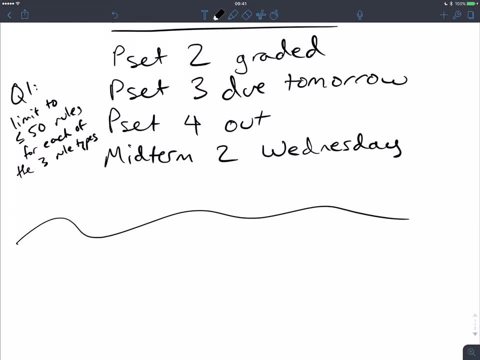 Yeah, If you happen to have fewer, like in the case of state, state goes to epsilon for the first rule type. if you have fewer than 50 states, you can't make 50 anyway. So yeah, At most 50.. 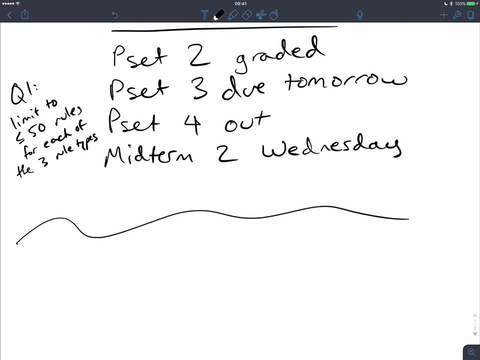 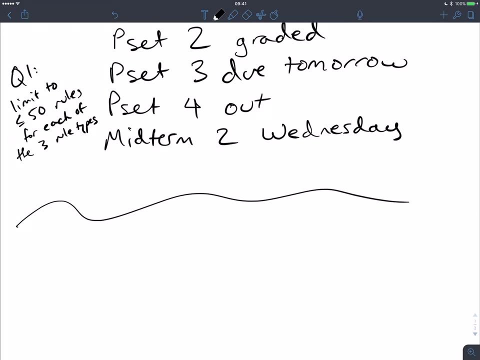 I mean, if you want to include the whole output, you can. But yeah, Any other questions about pset3?? Okay, Pset4 I posted, I think, this morning. So any questions about pset4? No, Okay. 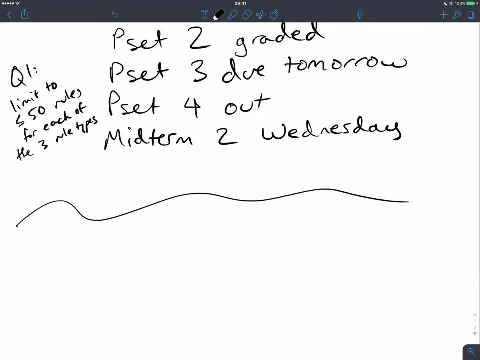 Okay, Okay, Okay Okay. Mid-term 2 is on Wednesday. Any questions about mid-term 2?? It covers well, it definitely covers up until the end of today, But in terms of material before I'm not going to explicitly ask about like information. 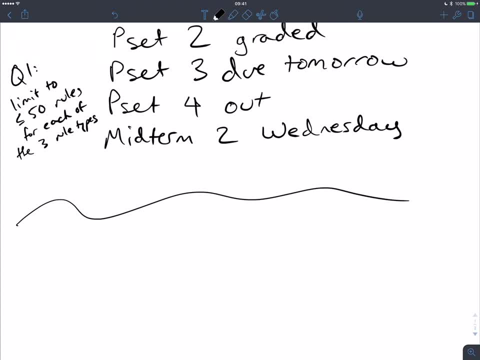 that was on mid-term 1. Like I'm not going to ask converted NFA to DFR, Okay, like I'm not going to ask that, but knowing like NFAs and DFAs are equivalent, that may or may not be important, like like the knowledge of that is important. 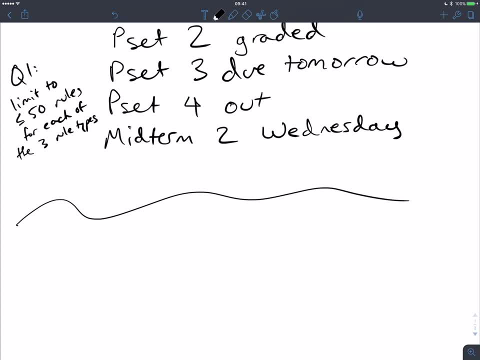 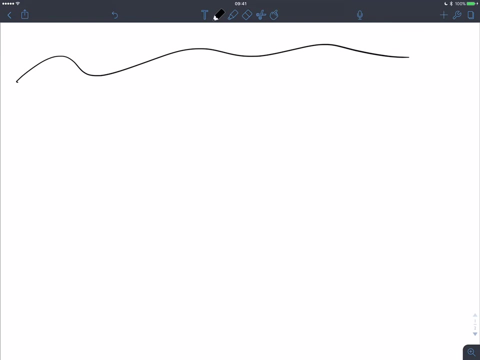 but not like actually doing the computation or whatever. that particular pumping one, I guess, the context free one, for sure, yeah, because that was past. any questions about midterm to that? okay, so where did we leave off on Friday? right? so we talked about this notion of decidability. so we say that a language was decidable if there's a Turing. 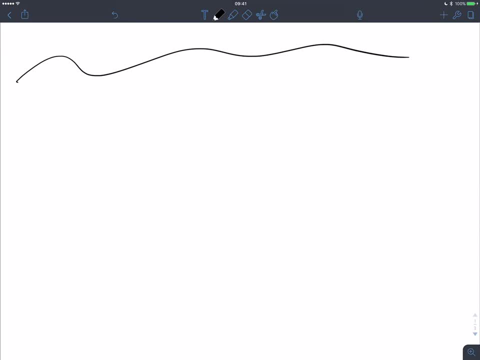 machine that, no matter what input it gets, it'll always stop on that input and say accept or reject, based off of what the language happens to be. and we've also saw that recognizable languages are those where you only had to halt on the strings in the language and say accept. 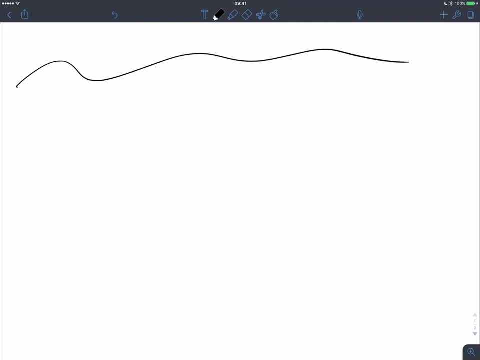 of course, but you're not required to hold on the ones not in the language. okay, and that'll turn out to be an important distinction. so, keeping along those lines, we were able to see various languages about. you know, the language itself and the language itself and the language itself. 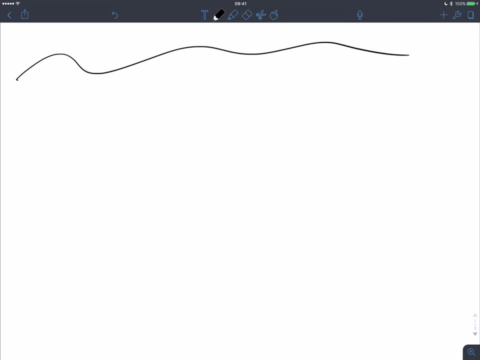 DFA's and NFA's that were decidable. so what languages did we see were decidable? yeah, ADFA and ANFA were examples. ADFA, we saw, was decidable because we could say, just run the machine on the input and since the computation must at each transition consume a character of the input, it. 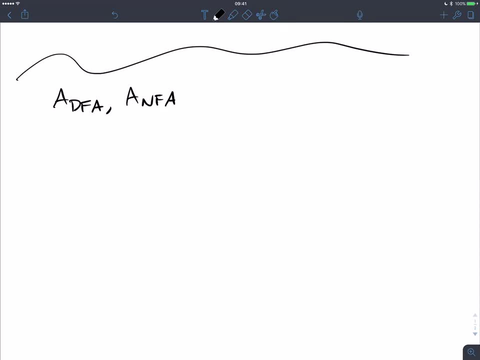 can't take an infinite amount of time to run a DFA on the input, and so, therefore, we could decide a NFA. we could decide a NFA instead of just simulating the NFA on the input, because, for two reasons, the turning machine is not non-deterministic, so it doesn't know. 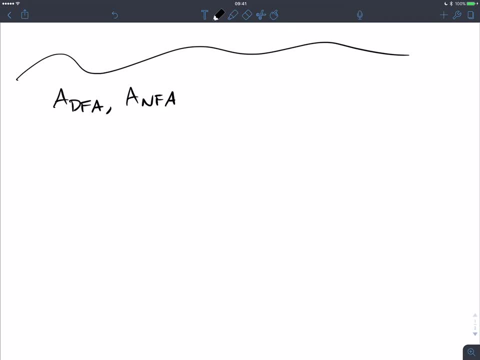 what choice to make. and even if it were, you could, for example, take a loop where you don't read any particular, any input at all. it's just a sequence of epsilon transitions and you never progress further. but we saw that if you convert the input NFA to a DFA, then run the decider for a DFA on the now DFA. now we 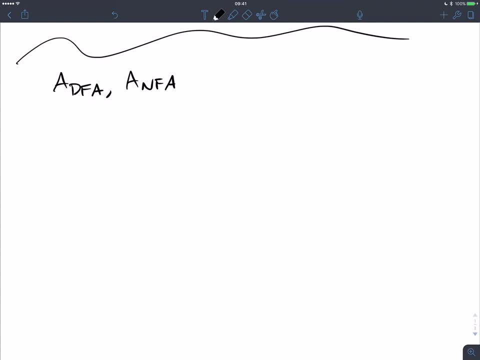 could decide a NFA, because the language of the DFA that's resulting is exactly the same as the NFA that was given to us. so we can decide a NFA. what about a REX and an ADFA? this is a pairs of R and X, where R is a REGX and X is described by that REGX. 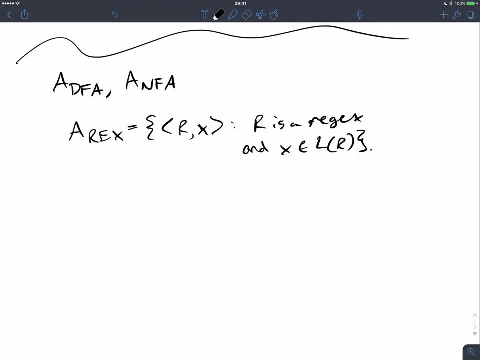 it's in the language bar is: yeah, why is it decidable? well, my task is: I'm given this REGX and I'm given this string and I'm my tasks is to determine if this REGX can make that string yeah, right, so can I decide a? 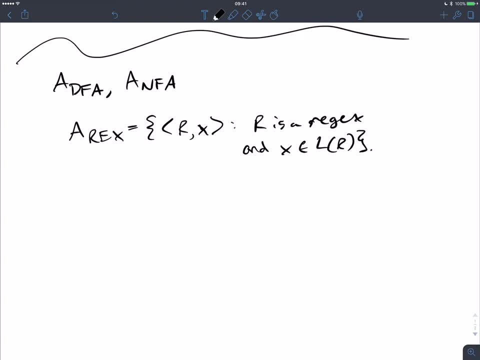 NFA. yeah, so is there something about REGX as an NFA that we know? they're equivalent because we can have a conversion between a REGX and an NFA. so to decide this, we take on input R and X, convert R into an equivalent NFA. 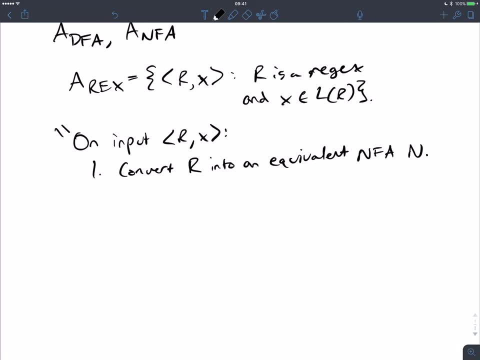 let's call it N. let's say: and then now, what should I do? right, run the decider. let's call that particular decider D for a NFA on. well, what two things does an NFA- sorry, a NFA's decider- expect a DFA from a REGX and an ADFA? 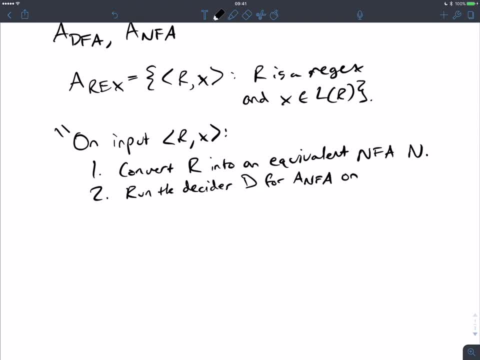 well, what two things does an NFA- sorry, a NFA's decider- expect a DFA from an ADFA as input- I'm NFA and a string. well, what NFA do I have N and what string do I have X? so I just feed it the pair N and X. so then, since D is a decider, then it. 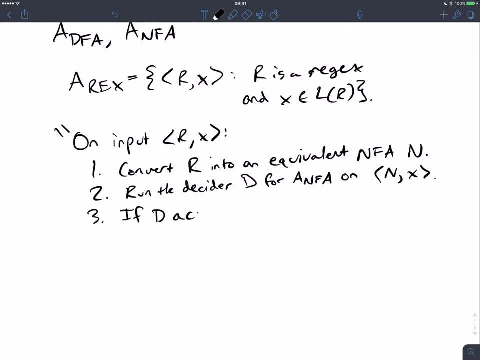 must say accept or reject. so D accepts, then that must have meant that the NFA accepted the input X. but that also means that the REGX must have would have described that string X anyway. so we should say: except here. and then the other case: if D rejects, that means the 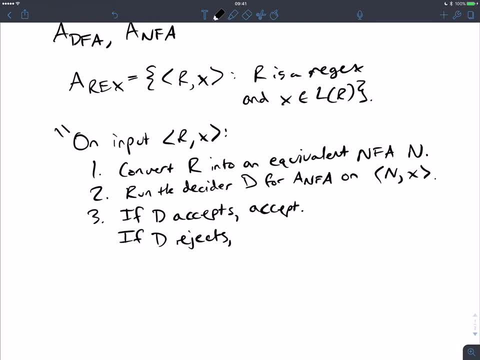 NFA did not accept the input X, which means the REGX R couldn't have described X anyway. so we say reject. the correctness is a pretty straightforward. but is this an actual decider or a REGX? does this run in a finite amount of time on all inputs? well, 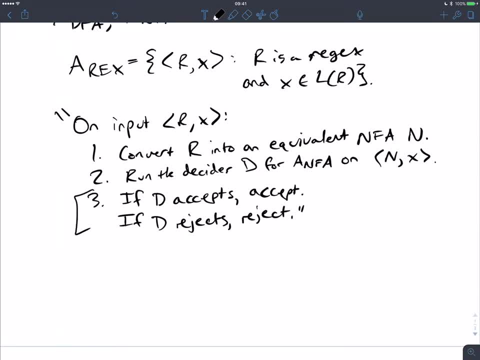 clearly, step three takes a finite amount of time. just step to take a finite amount of time. yeah why? because D is a decider. to step one take a finite amount of time. yeah why? because is an algorithm that works for any REGX and since the REGX is. 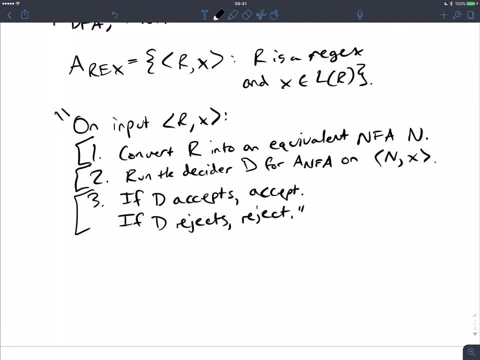 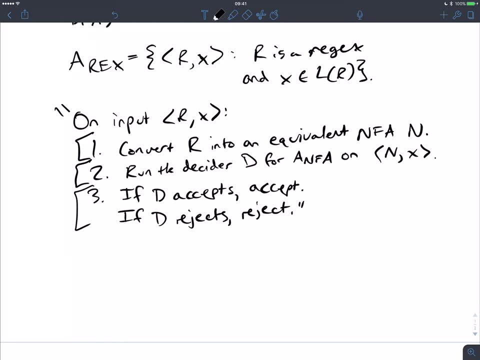 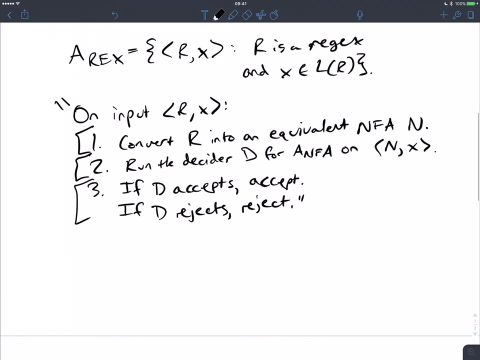 finite in size. the NFA that it produces is finite in size. okay, any questions about a REX. should have called it T-Rex. any questions, though You can't say that step two takes a finite amount of time because the string X is finite, right. 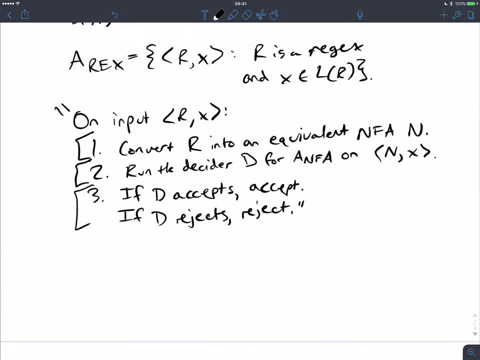 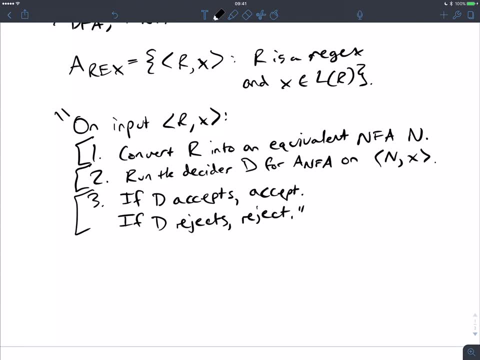 No, no, Yeah, yeah. well, the input is always finite, so there's never a problem there. the machine that we had for ANFA wasn't a decider. you have to go back to step two and we can't say that, except for the input, that was not finite. so the input is always finite. 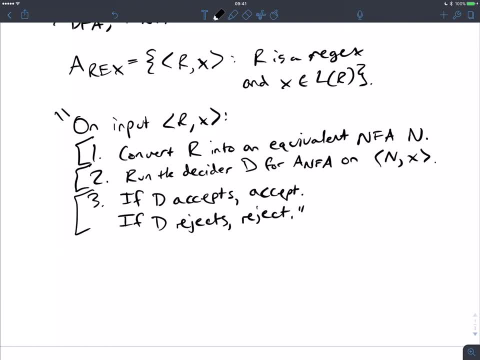 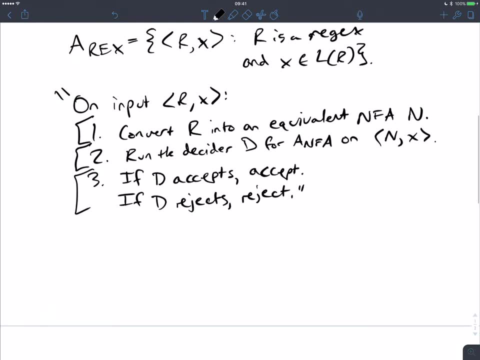 so there's never a problem there. the machine that we had for A-N-F-A wasn't a decider. yeah, all right. no, so should I say except for E-N-F-A, should I say except for decider? So, no matter what it got it halted. Yeah, Other questions? Okay, Well, so we actually 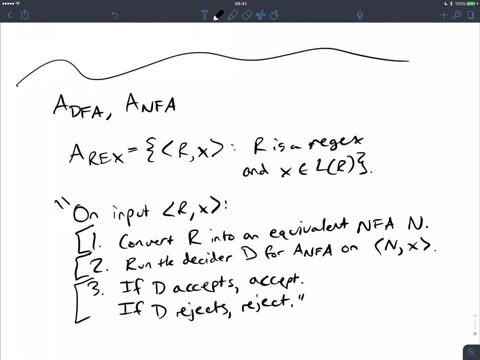 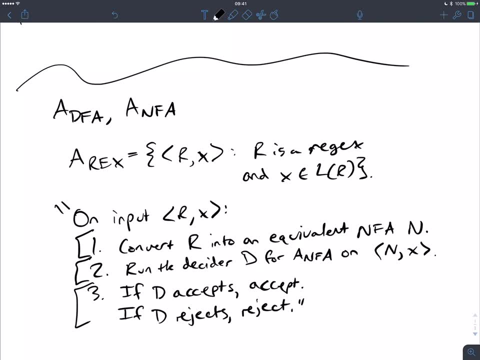 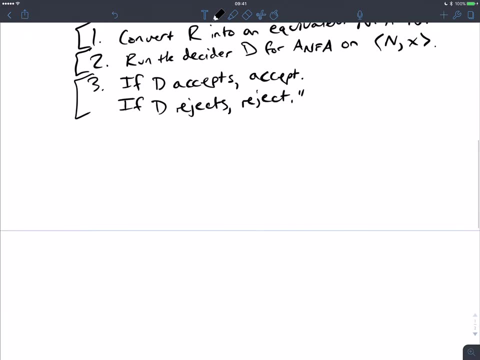 were able to show that all regular languages are decidable, because the problem of figuring out whether a string is in the language of some DFA, NFA or regex we just showed those problems are decidable. So all regular languages are decidable. So I want to take a little. 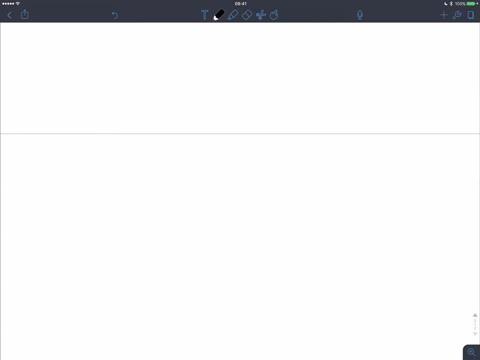 detour and talk about other languages that may be of interest. So I want to talk about one, and then we'll use that to solve a problem that we actually may want to solve ourselves. So the problem I want to talk about is called EDFA, So instead of A-NFA- sorry, ADFA it's. 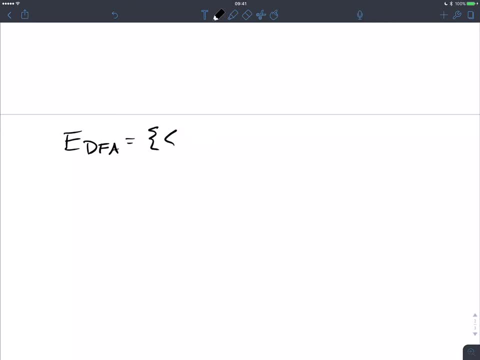 EDFA, And instead of a machine and a string, we're given exactly one machine and no string. And what I want to check is that the language of M is empty. Oh, I should say that M is a DFA. This would be very, very different. if it's not a DFA, Okay. 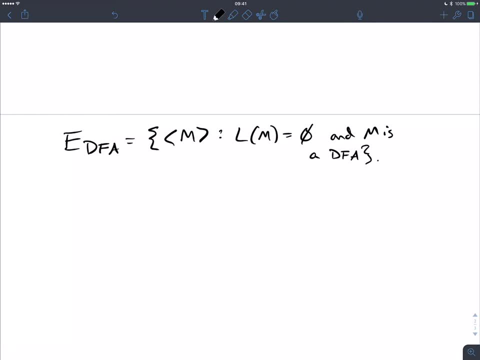 So instead of being given a machine and a string, I'm only given a machine here, no input at all. Okay, Well, no input string input machine. So if you have a DFA, you may want to figure out, does it actually do anything? So if I can show that this is decidable, then 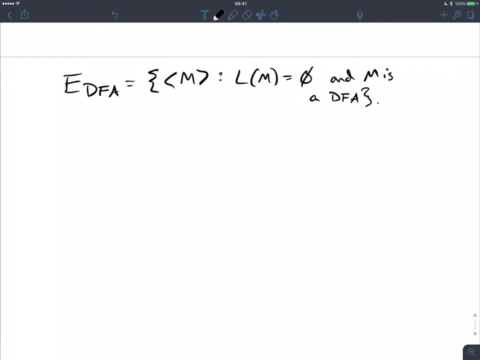 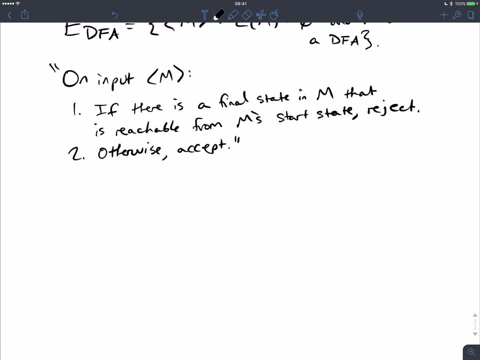 a DFA. what is a really easy way for you to figure that out? Well, if you are given good point, you should say in 0 or more transitions, because if it's reachable, a final state is reachable in 0 transitions. that is the start state. 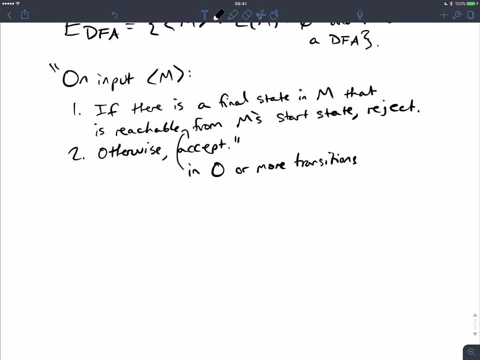 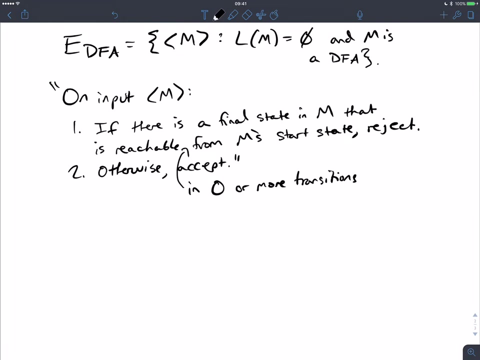 so that would cover that case. Reachable should mean any sequence of transitions, either empty or not. Question over here. A DFA is never decidable. Language is decidable. We're given any DFA. Well, that's actually not important here. I'm given a DFA and I need to check. 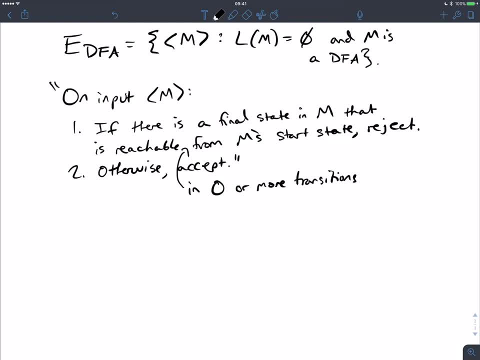 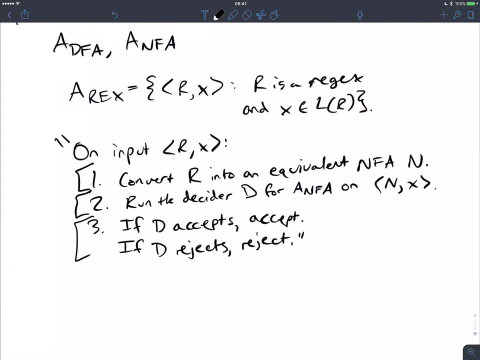 in a finite amount of time whether it accepts any string at all. Well, ADFA was the language of machine and string pairs, where M accepts that string, And so the problem there is just saying: can you check whether or not the machine accepts the input in a finite amount of time? 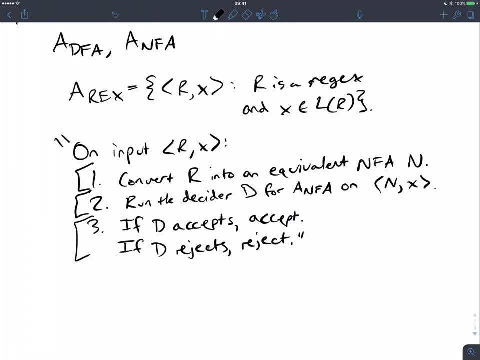 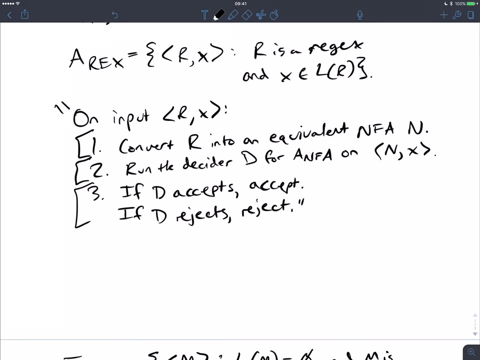 For any string. Yeah, for any string, any DFA- Well, there has to be one state. If it's a yeah, so this check at the beginning, right there, that checks if it's a valid input or not, Which you can definitely do in a finite amount of time. 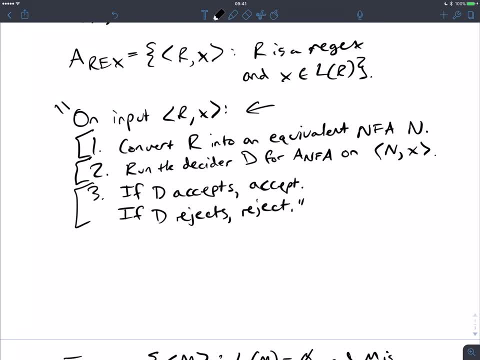 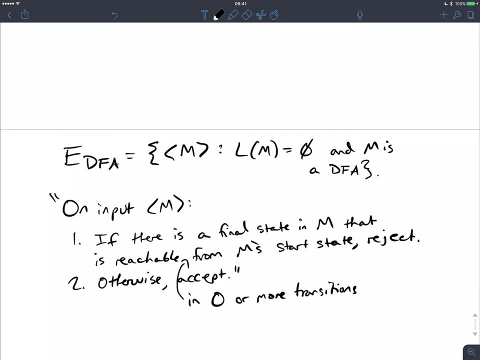 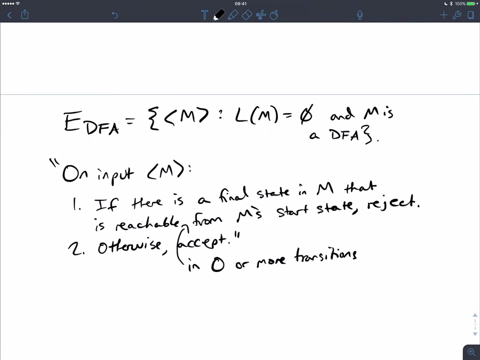 Okay, Yeah, Yep, You mean it runs in a finite amount of time? Yes, Yes, Yes, Yeah, And also justified correctness, for sure. But yeah, it has to run a finite amount of time. Yeah, Other questions: 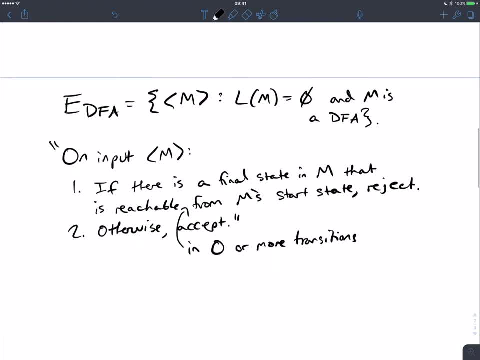 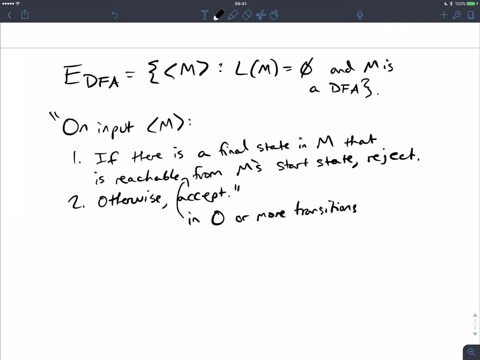 Okay, Cool. So any questions about EDFA Empty. Yeah, So we're going to see maybe three more examples of Es, Es of something? Yeah, What is the? A Accept, Accept Or acceptance? Yeah, It's just a name, but that's what it represents to us. 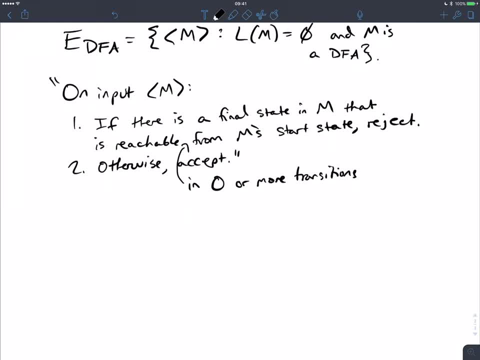 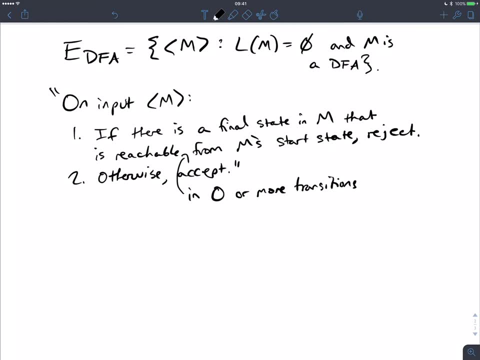 Okay, Okay. So one thing that is quite troubling about, say pset one, was that we asked you to present a DFA for a particular problem. Okay, Okay, Okay, Okay, Okay, Okay, Okay. And you said that you only know the sarcasm. 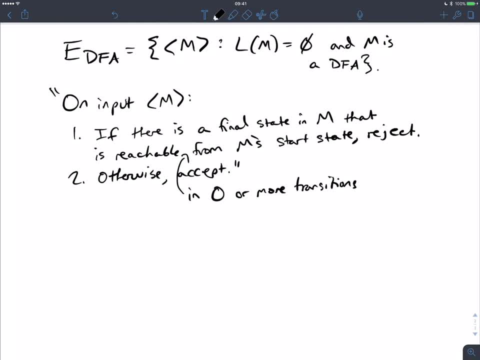 And that is like a major problem. It's not the kind of big talk that goes on within says as far as how much error you get from a problem And the poor grader has to figure out if the given DFA that's from your. 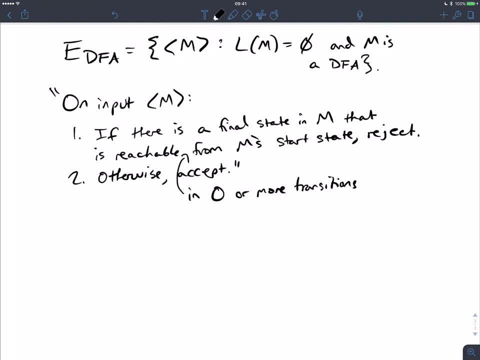 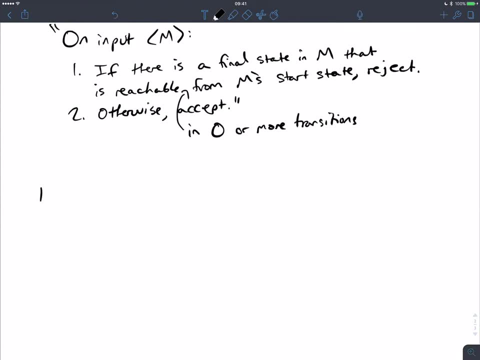 submission matches the input. sorry, the sample solution that we provide the grader And one may want to know: are these two DFAs actually the same out, whether they actually have the same language. So the problem I want to talk about next is EQ. 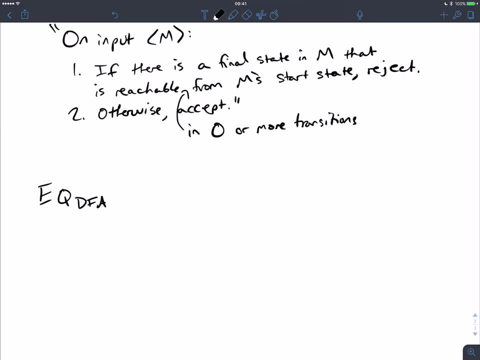 DFA, which means equivalence or equivalent DFAs. So instead of being given either a machine string pair or just a single machine, here we're given two DFAs. So I'm going to be given M1 and M2. so M1 and M2 are DFAs and they have the same language. 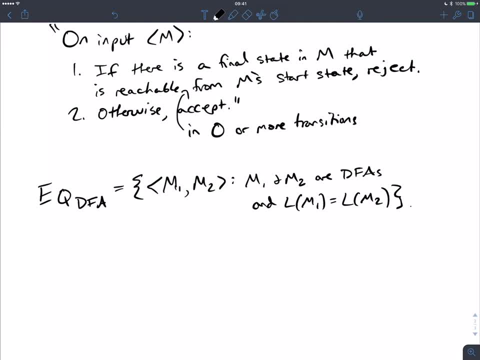 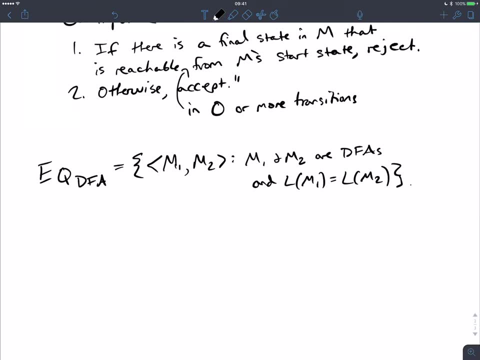 And certainly, if we want, if we can show that this is decidable, then we can actually write a computer program to figure that out, for us to figure out whether the two machines have the same DFA or not. So we can actually write a computer program to figure that out, for us to figure out whether the two machines have the same DFA or not. 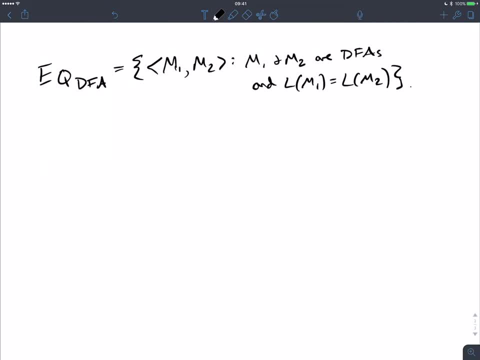 So we can actually write a computer program to figure that out, for us, to figure out whether the two machines have the same language or not. So how do you think we can do this? Any ideas? So here's a good idea: If you're tasked to prove that two things are equal. 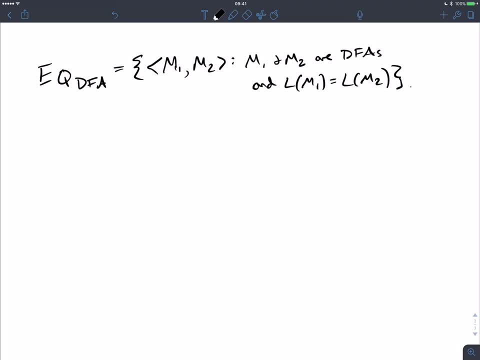 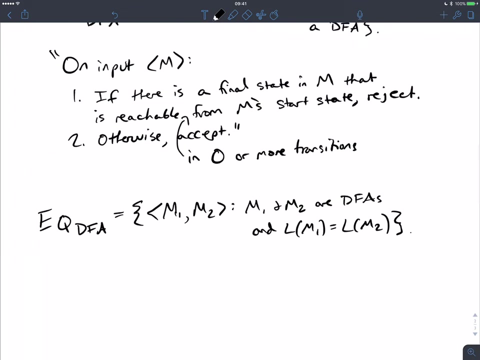 in this case, sets languages. how can you do that Exactly? If I can show that L of M1 is a subset of L of M2 and the other way around, are they equal? Okay, let's see. So I'm not going to actually write a whole algorithm like this, but 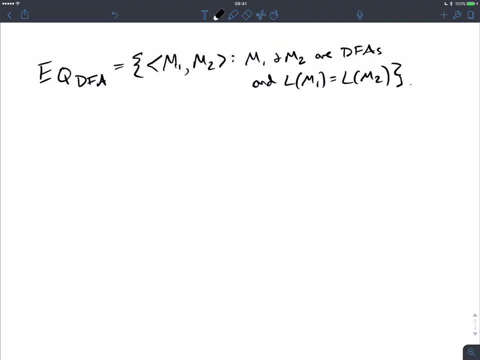 it's easily constructible from this. So this is the same as determining if L of M1 is a subset of M2.. So again, this is L of M2's language and L of M2 is a subset of M1's language. 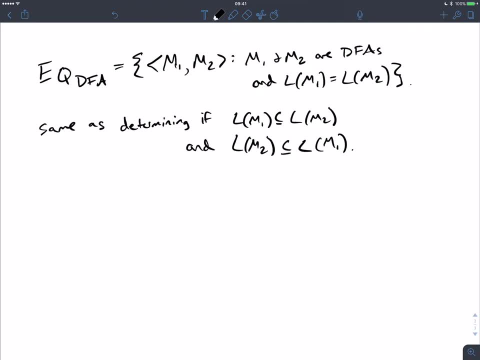 If we can do that, that's fantastic. What's another way to write? subset L is the language of N N is the subset of N N. So L of M2 is a subset of N N N. So a picture will help. 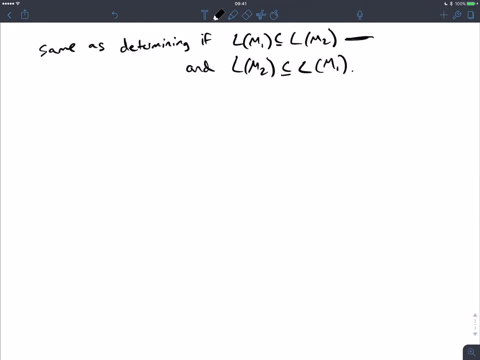 So let's just say that we're in this first case. So M1's language and M2's language may or may not be contained within one another. So let's say M1's here and let's say that there's some intersection in M2's out here. 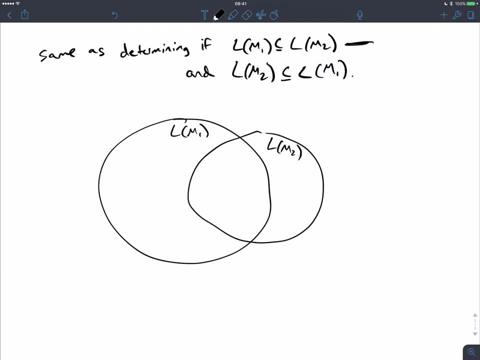 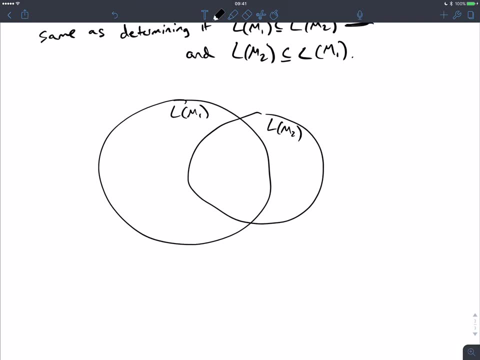 There may or may not be, I don't know. So in this particular example, M1's language is definitely not a subset of M2's language. So how do you know that it's not a subset? That's actually exactly what it is. but let's get a more intuitive idea. 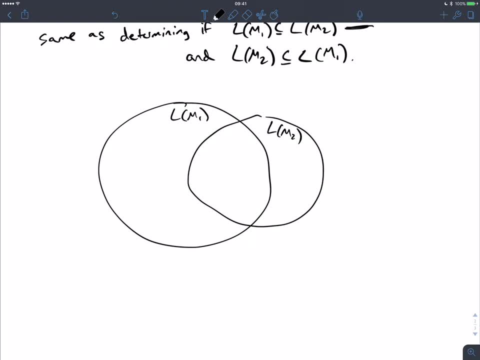 In this particular Venn diagram. what do we want to be? What do we want to be not there at all? Yeah, the stuff right here. We don't want this part to be present at all. In other words, I want this part to be empty, right. 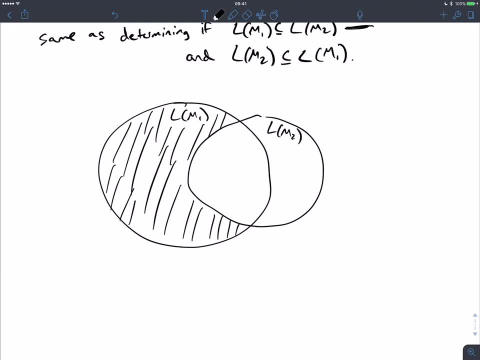 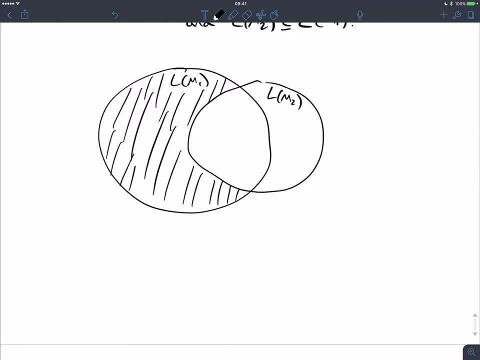 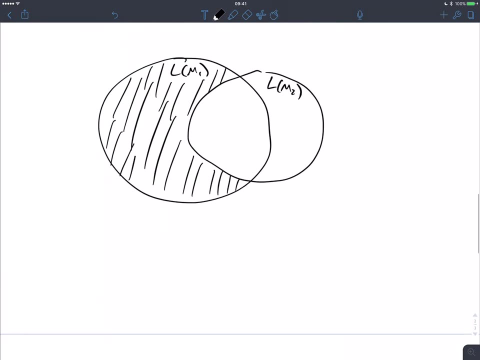 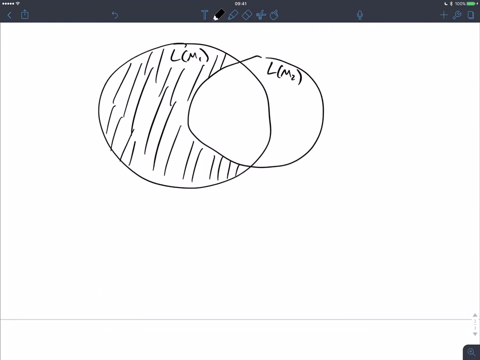 How do I represent that shaded area in terms of L of M1 and L of M2?? Well, let's see. Okay, Yeah, so it's. so. I want to talk about the actual area. So it's definitely in L of M1, but it's also not in L of M2.. 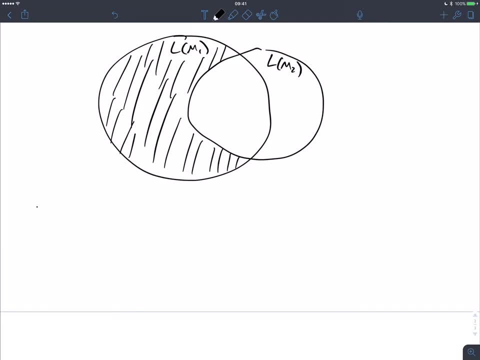 Yeah, yeah, So it's equal to L of M1 minus the complement of M2, but another way of writing, that is L of M1.. Intersection: Oh no, not the complement on the first one, L of M2 complement there. 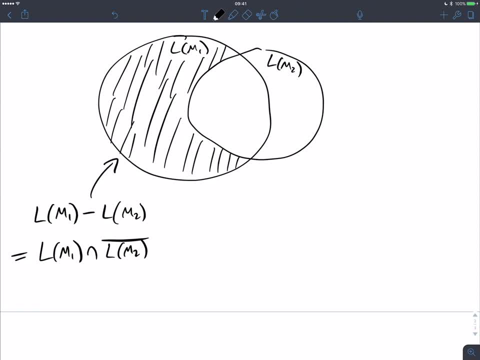 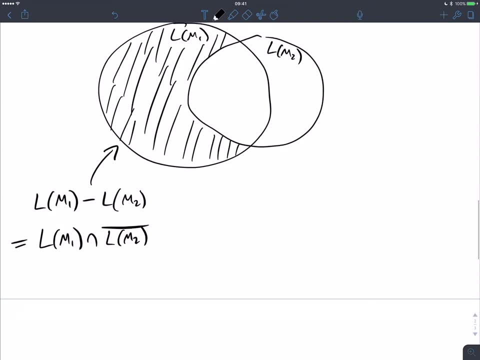 So I want everything. so that shaded area right there represents everything that's in M1, take away the things in M2's language, But another way of writing. that is the thing I wrote below, which is the things in M1's language and not in M2's language, which is just intersection. 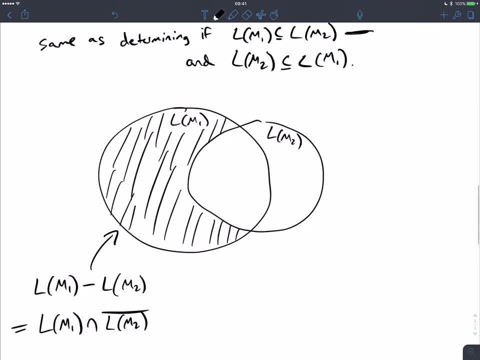 Okay, So conversely, for the second subset, what area do we want to be also empty? The part that belongs to M2 over here. I'm not the best at drawing or shading. Anything arts and crafts related, All right. 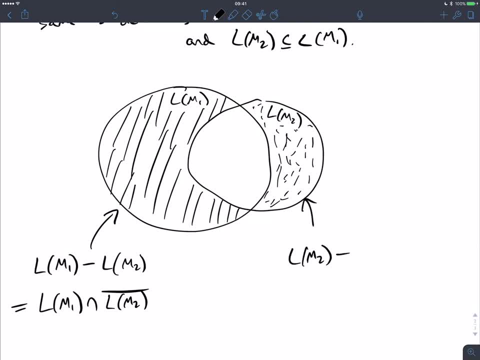 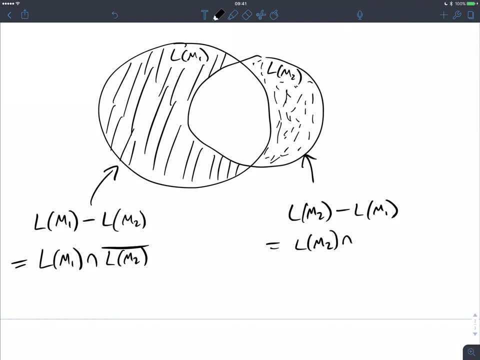 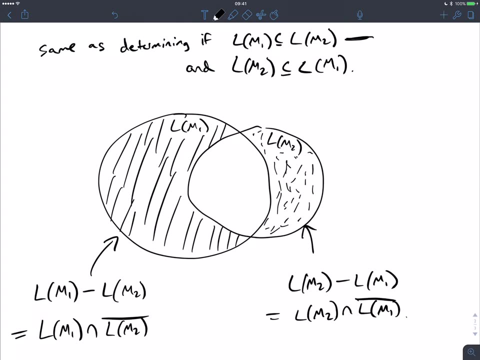 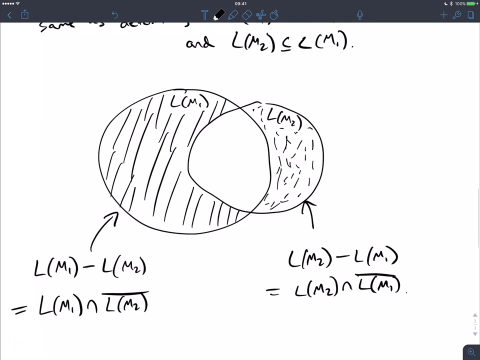 So this is just L of M2 without M1.. Which is just L of M2 intersect, M1 complement. Yeah, Yes, Great point. It is symmetric difference Because these are the strings that belong to exactly one or the other. All right, 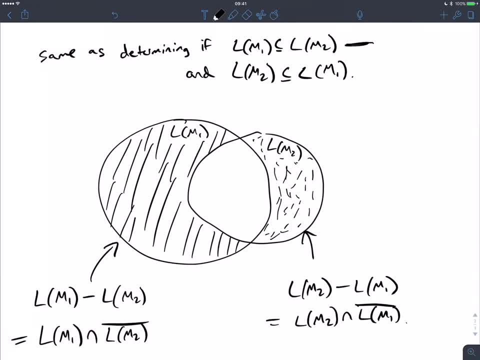 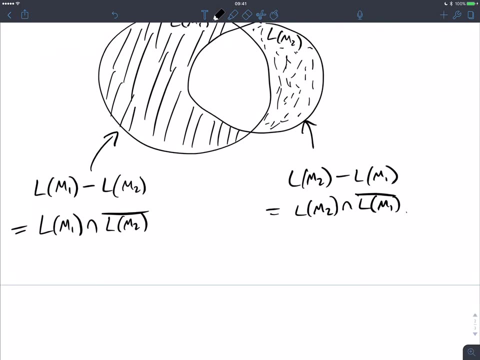 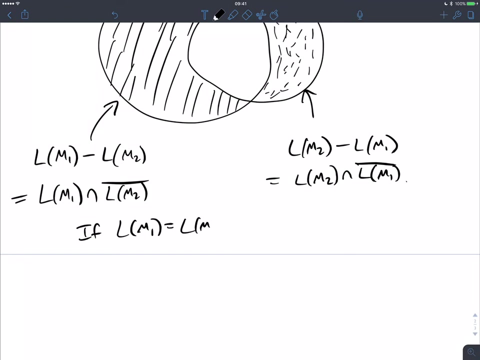 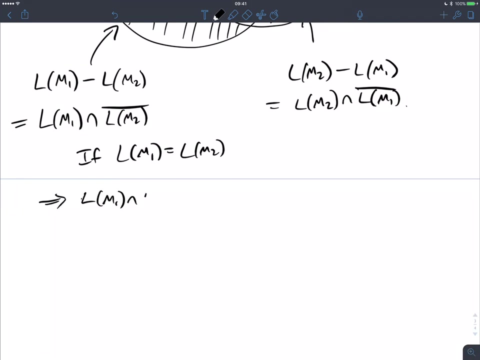 Well, If they're equal, What do I know about both? All right, of these regions, the shaded regions? they don't exist, so they're both empty, all right. well, if L of M 1 equals L of M 2, then this implies L of M 1 intersects L. 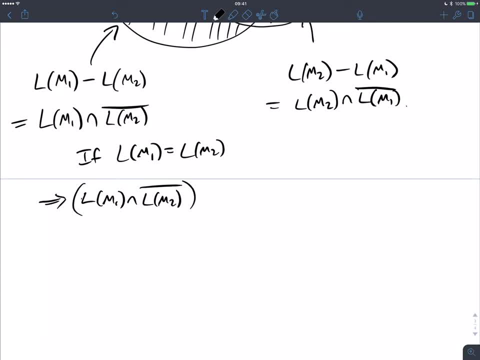 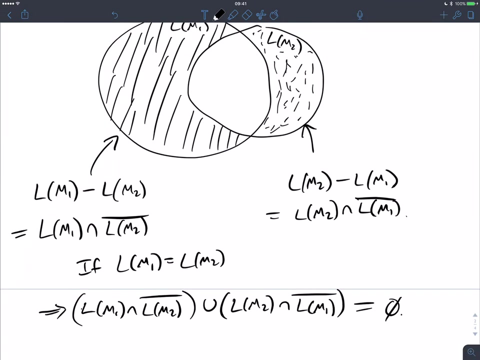 of M 2 compliment. so the first guy Union with the second one is empty. so if either one of these two is non-empty, then this Union is not empty. so if either one of these two is non-empty, then this Union is not empty. so if either one of these two is non-empty, then this Union is not empty. but if they're both empty, then the 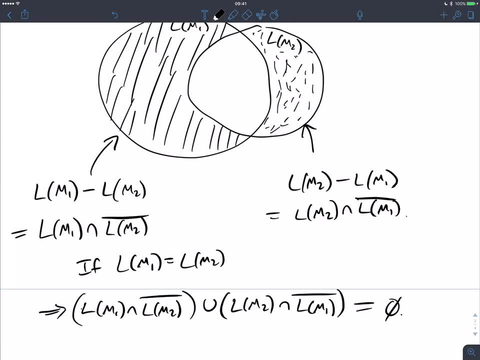 empty. but if they're both empty, then the empty, but if they're both empty, then the Union is empty. okay, so this is just a Union is empty. okay, so this is just a Union is empty. okay, so this is just a way of saying: if they're equal, then that. 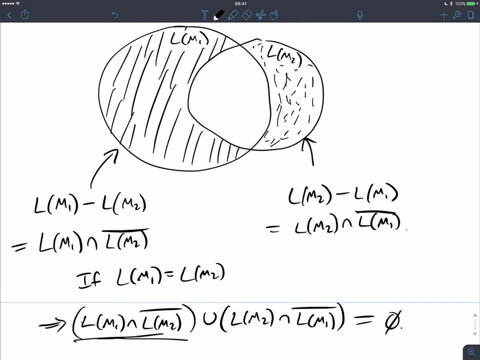 way of saying: if they're equal, then that way of saying: if they're equal, then that the first part must be empty and the the first part must be empty, and the the first part must be empty and the second part must also be empty. yeah, but I. 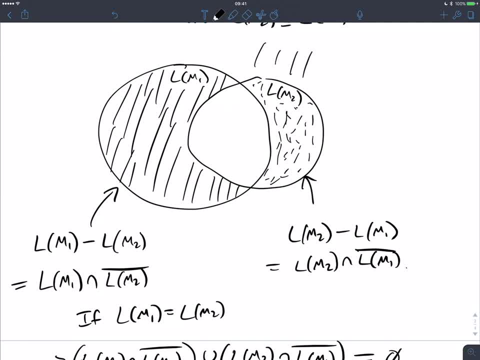 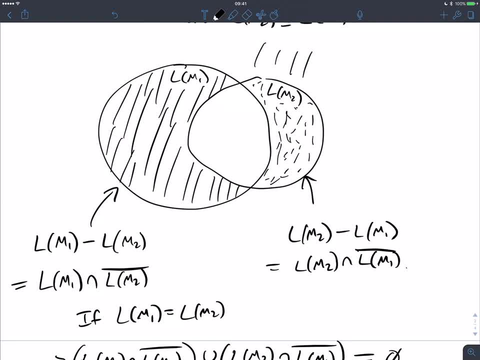 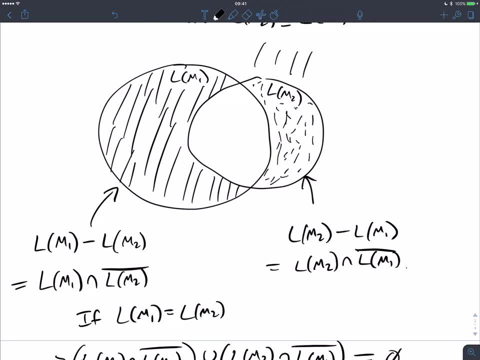 that's in L of m1 and L of m2, but also the stuff outside too, and I don't want the stuff outside too, and I don't want the stuff outside too, and I don't want any of that. well, what I could do is the: 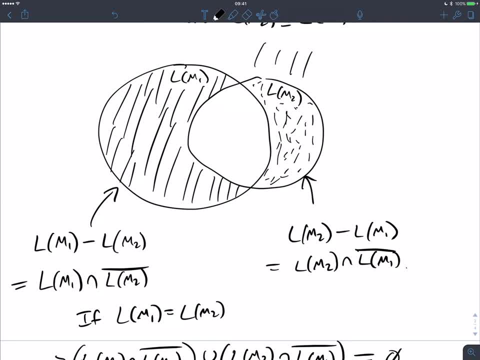 any of that. well, what I could do is the any of that. well, what I could do is the complement of the intersection. then take complement of the intersection, then take complement of the intersection, then take away the complement of the Union. that's away, the complement of the Union. that's. 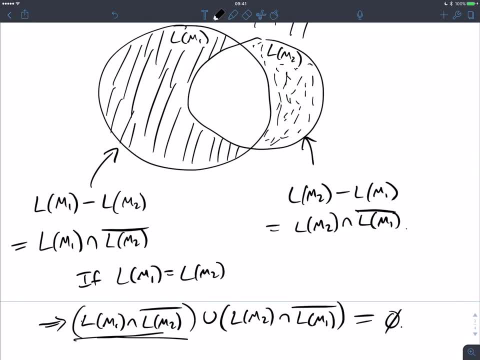 away the complement of the Union. that's another way of doing it. it's a but via another way of doing it it's a but via another way of doing it it's a but via De Morgan's laws is exactly the same as De Morgan's laws is exactly the same as. 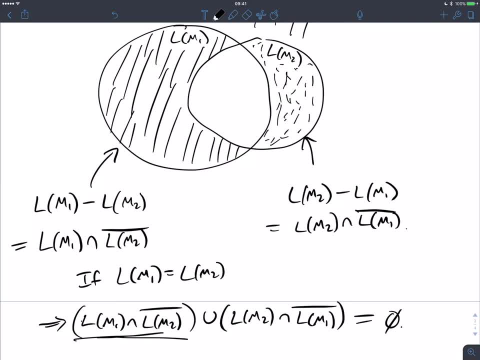 De Morgan's laws is exactly the same as this. yeah so. if yeah, so just the both this. yeah so. if yeah, so just the both this. yeah so. if yeah, so just the both parts of the Union. just say that I want parts of the Union. just say that I want. 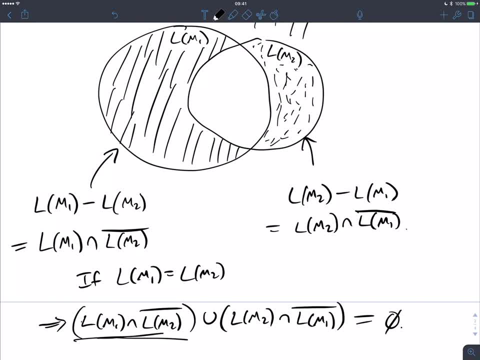 parts of the Union. just say that I want both of these two regions to be empty, both of these two regions to be empty, both of these two regions to be empty. okay, well, can I build a DFA for this? okay, well, can I build a DFA for this? 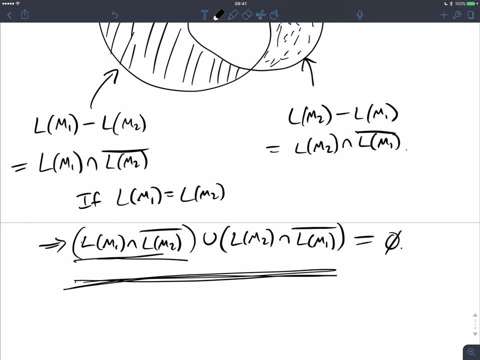 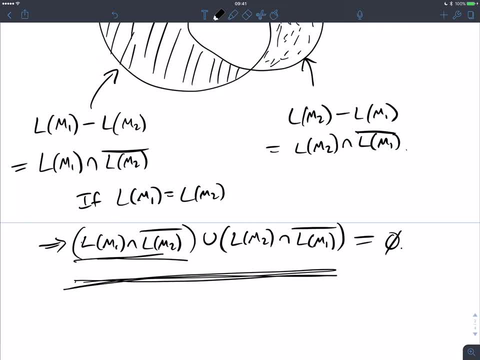 complement. okay, well, I can build a DFA for that part. could I check whether that for that part? could I check whether that for that part? could I check whether that resulting DFA's language is empty? yeah, resulting DFA's language is empty. yeah, resulting DFA's language is empty. yeah, why, we just proved that EDFA is. 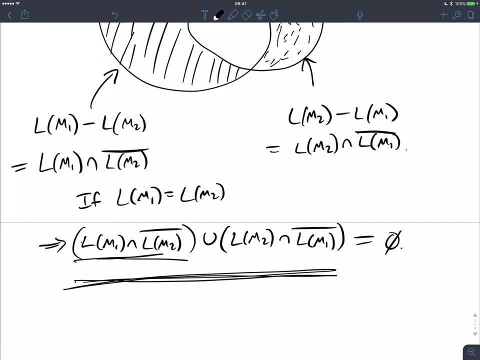 why we just proved that EDFA is why we just proved that EDFA is decidable, and so, therefore, I can do this decidable, and so, therefore, I can do this decidable and so, therefore, I can do this check. I didn't say that was the fastest. 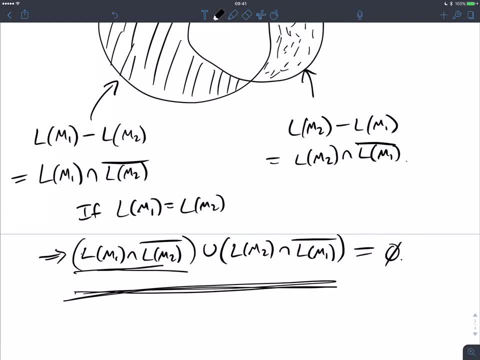 check. I didn't say that was the fastest check. I didn't say that was the fastest algorithm. I didn't say was efficient algorithm. I didn't say was efficient algorithm. I didn't say was efficient or pretty. I'm just saying that you can do or pretty, I'm just saying that you can do. 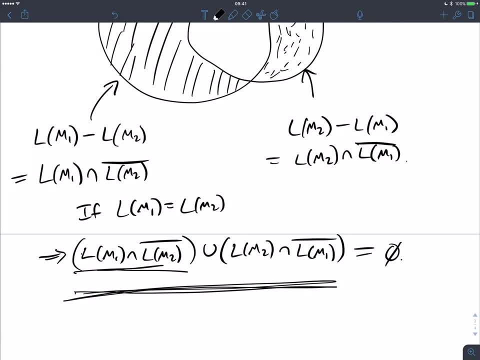 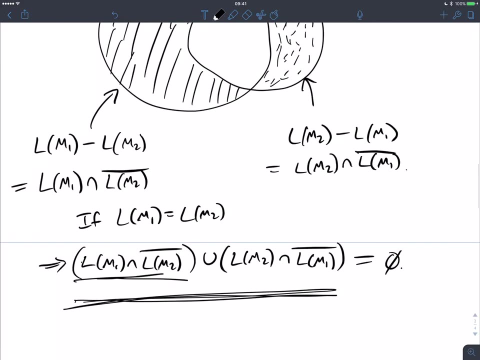 or pretty. I'm just saying that you can do it. yeah, no, I should have wrote a it. yeah, no, I should have wrote a it. yeah, no, I should have wrote a program but no middle. yeah, they in theory program, but no middle. yeah, they in theory program, but no middle, yeah, they in theory. could any questions about EQ? DFA is EQ. 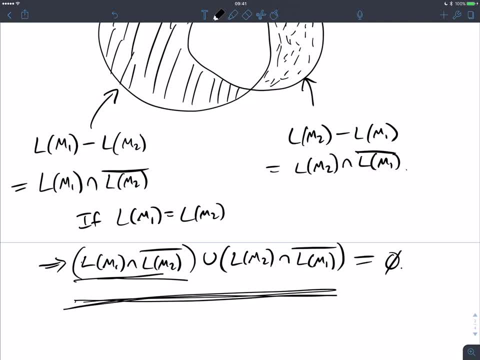 could any questions about EQ? DFA is EQ. could any questions about EQ: DFA? is EQ? NFA decidable? yeah, how just convert to a NFA decidable? yeah, how just convert to a NFA decidable? yeah, how just convert to a DFA? run that out, DFA. run that out. 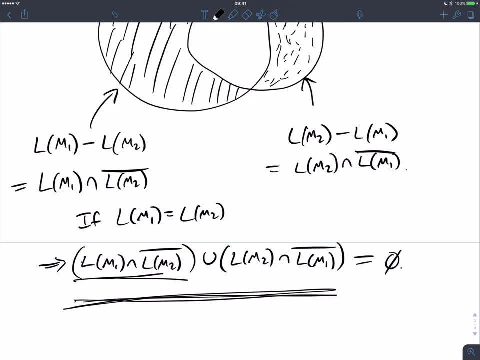 DFA, run that out with them. so we can get equivalents of with them. so we can get equivalents of with them, so we can get equivalents of regular expressions, regular grammars, regular expressions, regular grammars, regular expressions, regular grammars. anything with the regular languages, anything with the regular languages. 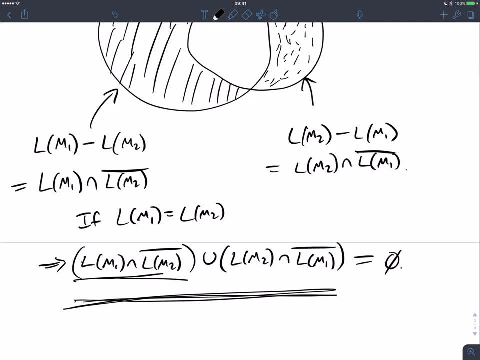 anything with the regular languages seems to be decidable, or testing for seems to be decidable, or testing for seems to be decidable, or testing for emptiness any of that's decidable. I emptiness any of that's decidable. I emptiness any of that's decidable. I want to do another one, and then I'll. 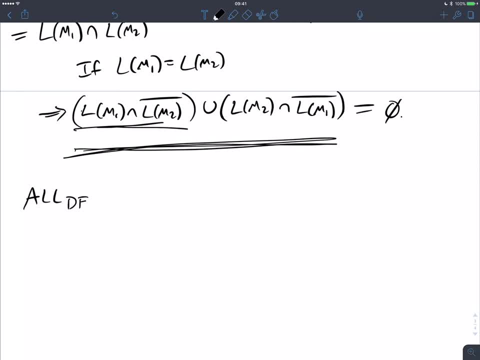 want to do another one, and then I'll want to do another one, and then I'll actually talk about a very interesting, actually talk about a very interesting, actually talk about a very interesting question right after that. so I call it question. right after that, so I call it. 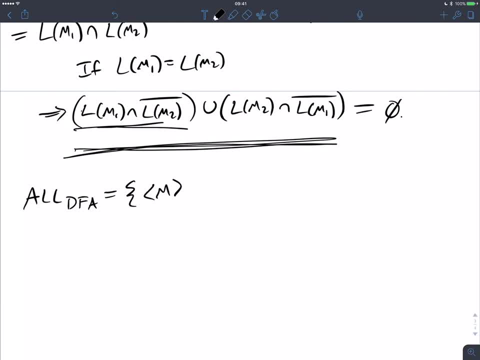 question right after that. so I call it all DFA. so we're back to a single, all DFA. so we're back to a single, all DFA. so we're back to a single machine and there's a DFA and it accepts machine. and there's a DFA and it accepts. 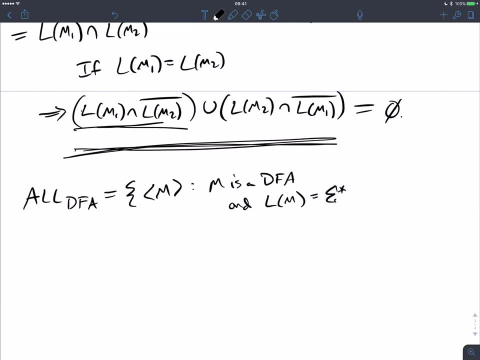 machine and there's a DFA and it accepts everything, every string. so there are everything, every string. so there are everything, every string. so there are actually two approaches we can take for actually two approaches we can take for actually two approaches we can take for this one. so how can I check if a DFA's 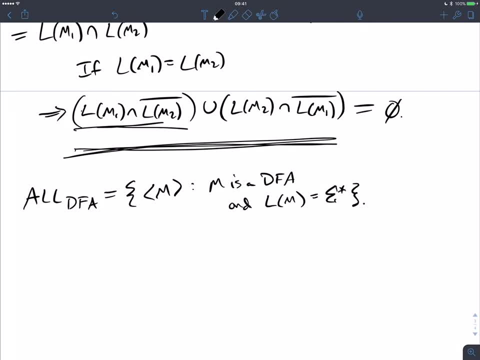 this one. so how can I check if a DFA's this one? so how can I check if a DFA's language? is every single string language? is every single string language, is every single string? any ideas? well, they're infinitely many. any ideas, well, they're infinitely many. 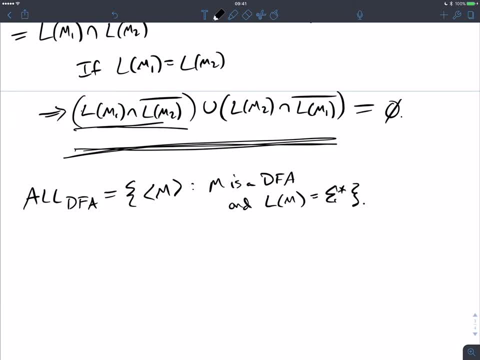 any ideas. well, they're infinitely many. strings. yeah, so, basically like that. strings, yeah so, basically like that. strings, yeah so, basically like that. every state that I could reach from the, every state that I could reach from the, every state that I could reach from the start state, is a final state, so that's. 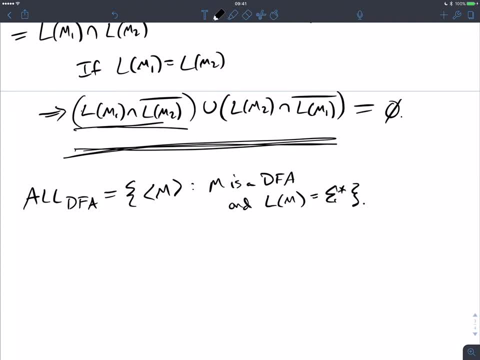 start state is a final state, so that's start state is a final state. so that's one way including yeah, every. just like one way including yeah, every. just like one way including yeah, every. just like before what's another thing, another way before what's another thing, another way. 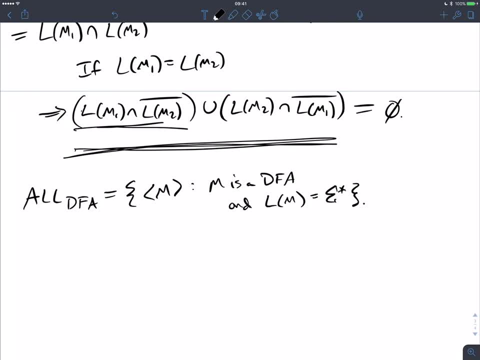 before. what's another thing, another way we can approach this. we can approach this. we can approach this if the DFA that's given to me really does, if the DFA that's given to me really does, if the DFA that's given to me really does accept everything. what is the? 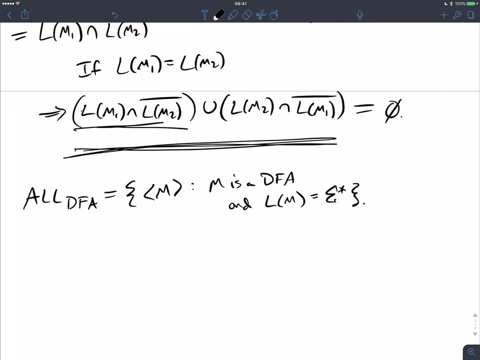 accept everything. what is the accept everything? what is the complement of that language empty? what complement of that language empty? what complement of that language empty? what if it wasn't everything when it was, if it wasn't everything when it was, if it wasn't everything when it was given to me? what is the compliment? it's? 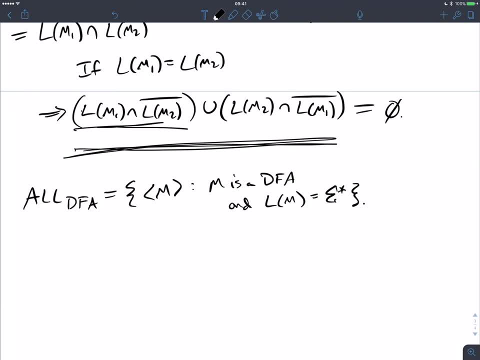 given to me. what is the complement? it's given to me. what is the complement? it's not empty. do we have a way of checking, not empty. do we have a way of checking, not empty? do we have a way of checking for emptiness? yeah, yeah. so so the first. 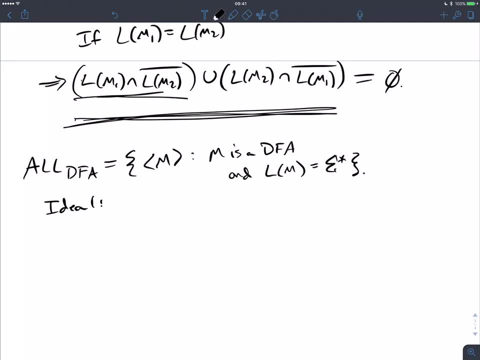 for emptiness? yeah, yeah, so so the first for emptiness. yeah, yeah, so. so the first idea is run. similar idea is run. similar idea is run. similar algorithm for EDFA, but invert final algorithm for EDFA, but invert final algorithm for EDFA, but invert final, non-final states, because it's a DFA here. 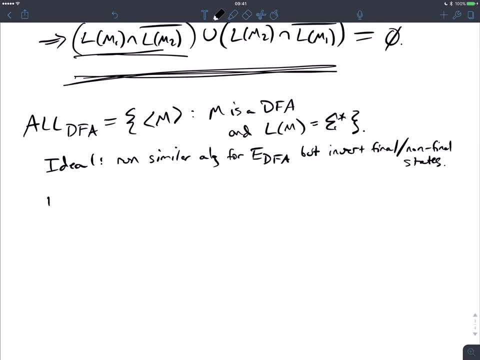 non-final states because it's a DFA here, non-final states because it's a DFA here. that's the only way. that's the only. that's the only way. that's the only, that's the only way. that's the only reason it works. but the other idea was: 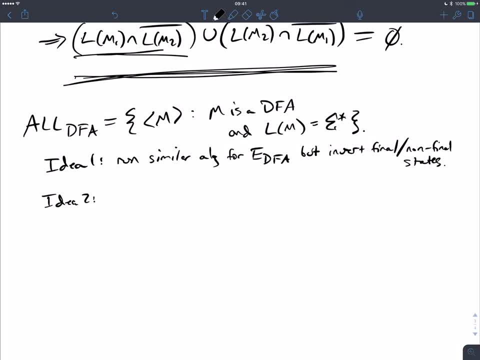 reason it works. but the other idea was reason it works. but the other idea was to: oh, I did it backwards. idea two was to to: oh, I did it backwards. idea two was to to: oh, I did it backwards. idea two was to check, check, check. no, I wrote this. I wrote both of them in. 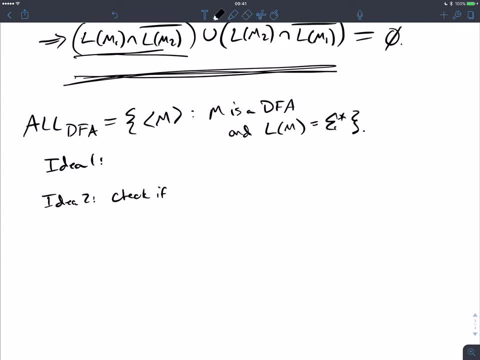 no, I wrote this. I wrote both of them in. no, I wrote this. I wrote both of them in one statement. all right, all right. so the one statement all right, all right, so the one statement, all right, all right. so the idea one is: check if the compliment, if 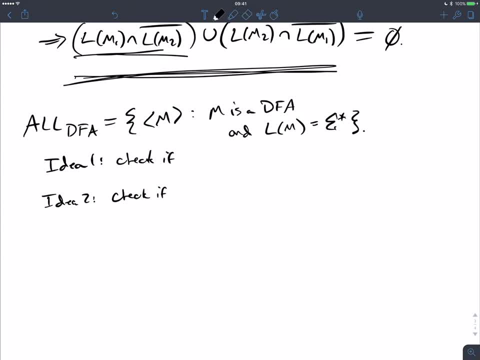 idea one is check if the compliment if idea one is check if the compliment. if every fall apart here. if every reachable every fall apart here. if every reachable every fall apart here. if every reachable state from the start status final and state from the start, status final. and. 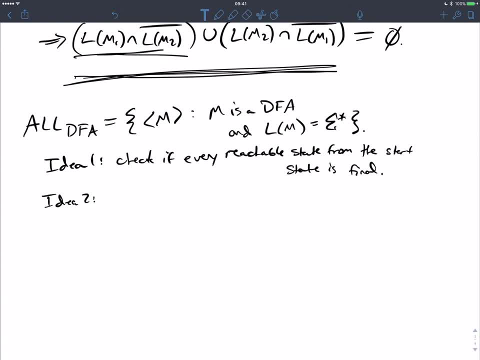 state from the start status final, and then the other one is invert final, and then the other one is invert final and then the other one is invert final and non-final states and non-final states and non-final states and check for emptiness. that's what I meant. 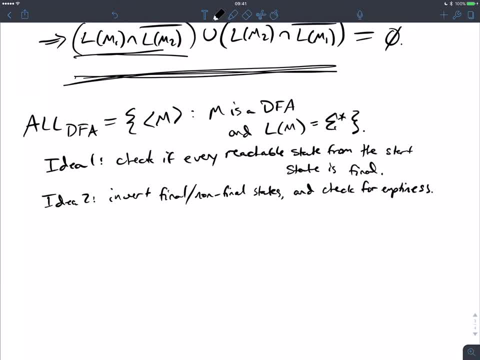 check for emptiness. that's what I meant. check for emptiness, that's what I meant- to write back. so either just check if to write back, so either just check if to write back. so either just check if every single state you could reach is. every single state you could reach is. 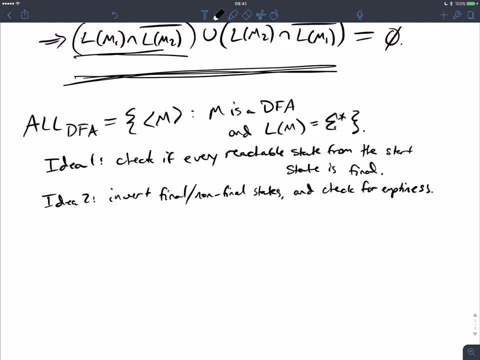 every single state you could reach is final, or just swap final and non-final final, or just swap final and non-final final, or just swap final and non-final for complement, as we've seen before, and for complement, as we've seen before, and for complement, as we've seen before, and run the decider for EDFA on the. 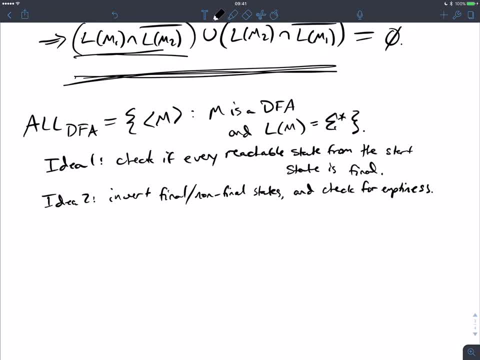 run the decider for EDFA on the run the decider for EDFA on the resulting DFA: either method. they're resulting DFA, either method. they're resulting DFA, either method. they're actually exactly the same method, but actually exactly the same method. but actually exactly the same method, but they seem to be different approaches. 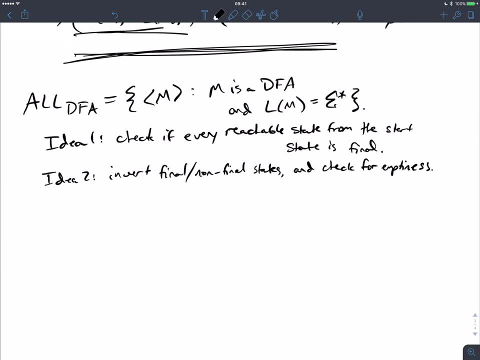 they seem to be different approaches. they seem to be different approaches. okay, the decider for EDFA? yeah, so check. okay, the decider for EDFA? yeah, so check. okay the decider for EDFA? yeah, so check, for emptiness means just run the decider. 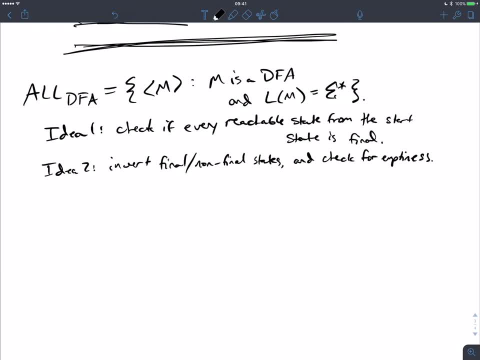 for emptiness means just run the decider for emptiness means just run the decider for EDFA. okay, any questions about all for EDFA. okay, any questions about all for EDFA. okay, any questions about all DFA. so you may think, well, okay, DFA. so you may think, well, okay. 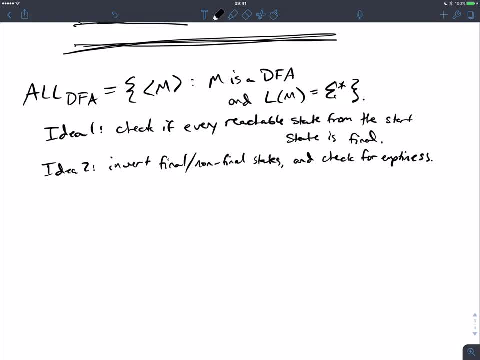 DFA. so you may think: well, okay, everything is decidable for DFA as it. everything is decidable for DFA as it. everything is decidable for DFA, as it seems like it seems like. seems like, it seems like. seems like it seems like it seems like. seems like it seems like all this theory about DFA's was solved a. 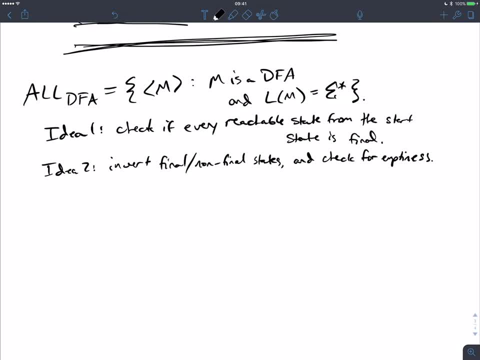 all this theory about DFA's was solved a all this theory about DFA's was solved a long time ago and we're just building up long time ago and we're just building up long time ago and we're just building up to eventually we show a language is not? 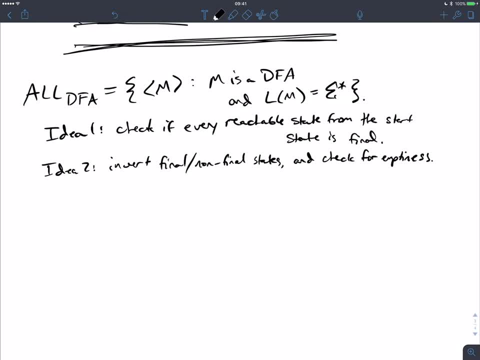 to eventually we show a language is not to eventually we show a language is not decidable. but everything about DFA's decidable, but everything about DFA's decidable. but everything about DFA's seems to be decidable, right, actually, seems to be decidable, right actually. 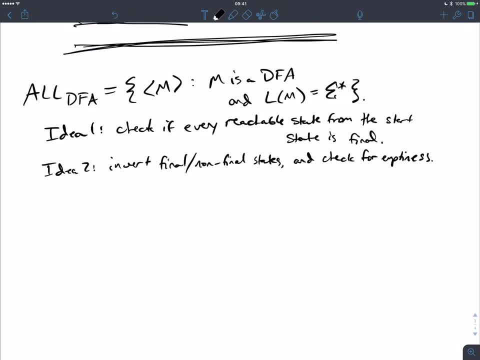 seems to be decidable, right. actually, there's actually one language that I know. there's actually one language that I know. there's actually one language that I know of that people still don't know whether of that. people still don't know whether of that, people still don't know whether it is decidable or not. about DFA's. 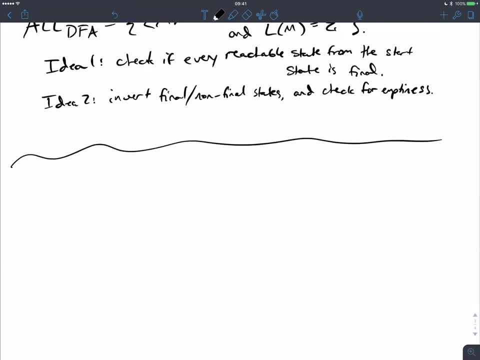 it is decidable or not about DFA's. it is decidable or not about DFA's, believe it or not. and it's this guy so believe it or not. and it's this guy so believe it or not. and it's this guy so. I mean I could put this on a homework. 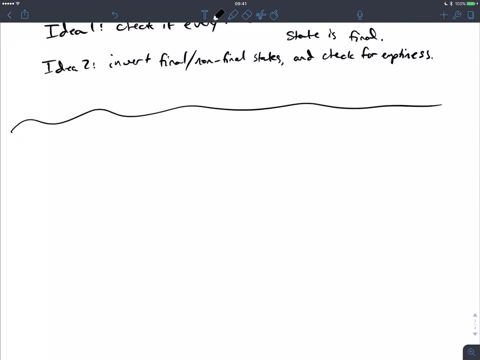 I mean I could put this on a homework. I mean I could put this on a homework, but it's an open research problem, so I but it's an open research problem, so I but it's an open research problem, so I won't. I'll be nice to you. so I want I. 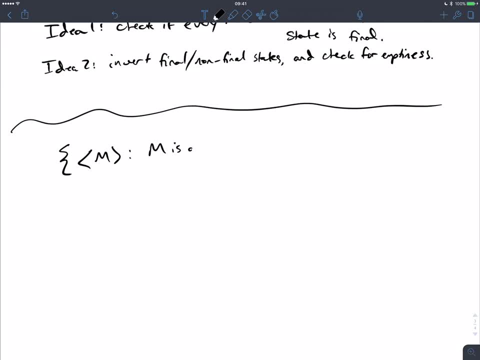 won't. I'll be nice to you, so I want. I won't. I'll be nice to you, so I want. I want all DFA's M, so I'll note that this. want all DFA's M, so I'll note that this. want all DFA's M. so I'll note that this is open. M is a DFA with alphabet. 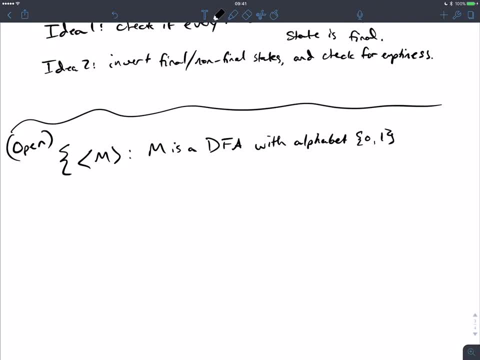 is open. M is a DFA with alphabet is open. M is a DFA with alphabet 0-1. so we're starting off nice and 0-1. so we're starting off nice and 0-1. so we're starting off nice. and accepts at least one string. 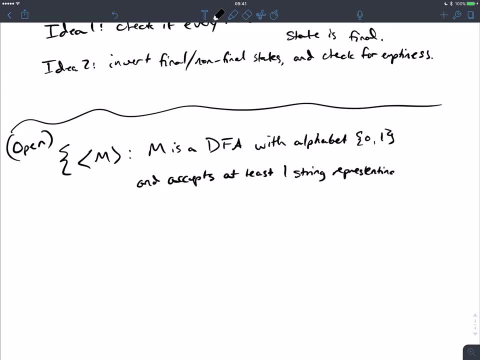 accepts at least one string. accepts at least one string representing a prime number. so I'll put this out as a bounty. so I'll put this out as a bounty: If you can figure out whether this language is decidable or not, you instantly get an A-plus in the class. 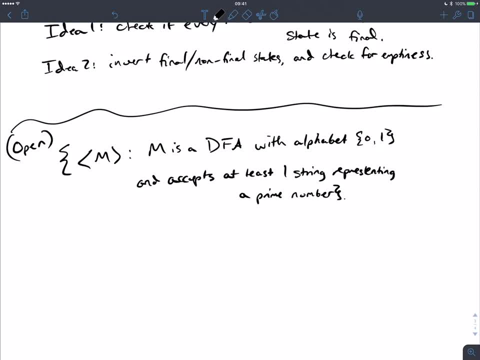 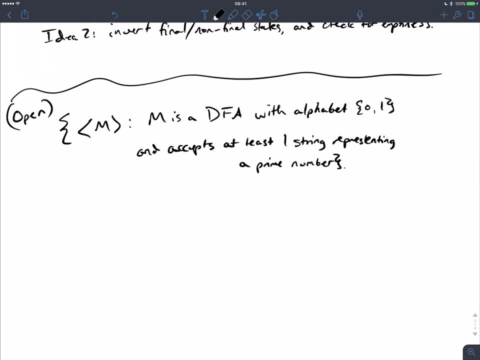 I'm not kidding about that, But I actually don't know what a good method to do this is. Can you show that this is recognizable? So here's an idea: Just enumerate the prime numbers in binary and then just check for each one whether the input DFA accepts it or not. 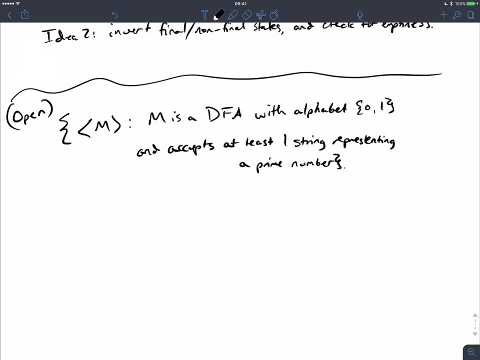 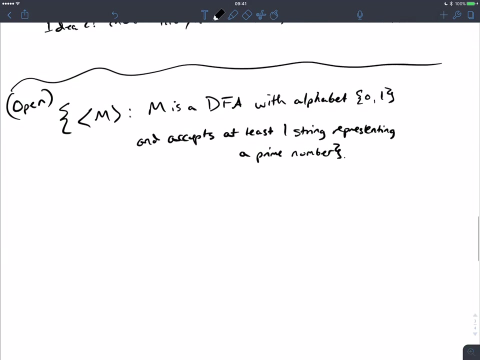 If it ever does accept a prime number representation, then I say accept. But can you show that if you do this strategy, you will never accept a prime number, And I don't know the answer to that. So open problem: A-plus if you solve it. 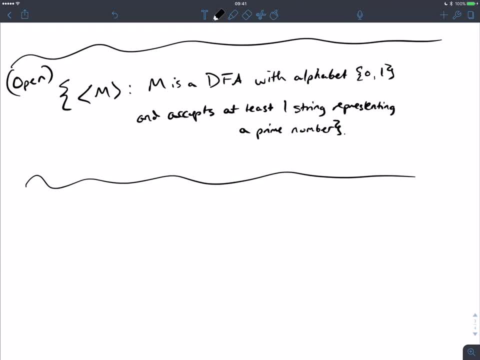 So it turns out, even today there are a lot of people who are using this method, But there are still open research problems about DFAs And it's going to get much worse once we go into the context-free languages. Any questions before we move on. 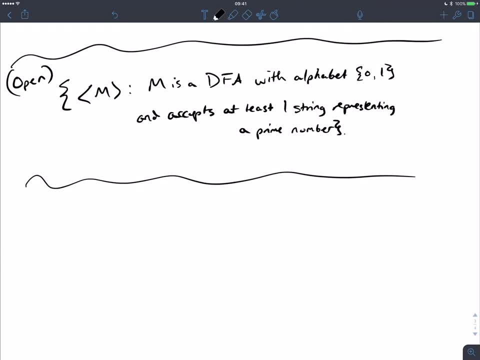 Okay, so when we first talked about decidable languages for DFAs, we talked about ADFA and ANFA, all that stuff. Then we talked about the emptiness question for DFAs, NFAs, whatever. Then we did equivalence And then we did: does it accept everything or not? 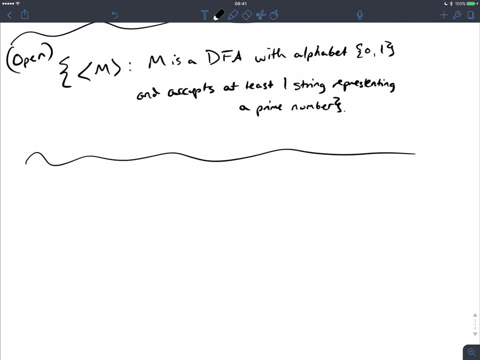 So let's start off easy for the context-free languages. So let's talk about ACFG. So instead of a machine and an input, it's a grammar and an input. So G is ACFG And W is generated by G. So draw my Gs better. 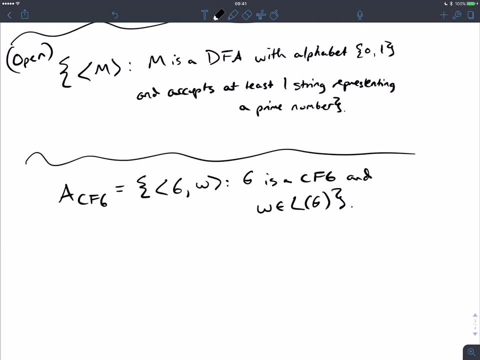 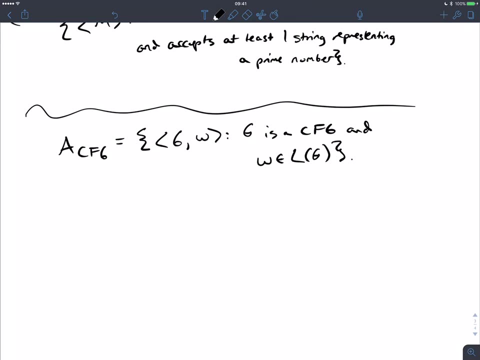 Okay. So you may think, well, ADFA was totally useless, right? This is actually really important. this language, ACFG, Because if you want to implement your compiler as a context-free grammar, that's just saying: well, I'm going to use this language as a context-free grammar. 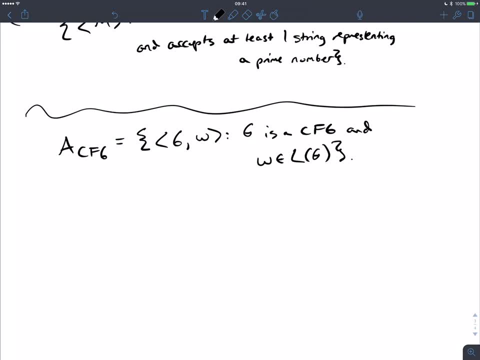 That's just saying your program compiles or not. Okay, So if it's in the language of your particular compiler, then this problem will help you solve that. Okay, So how could we show that ACFG is decidable? Well, it seems kind of hard right. 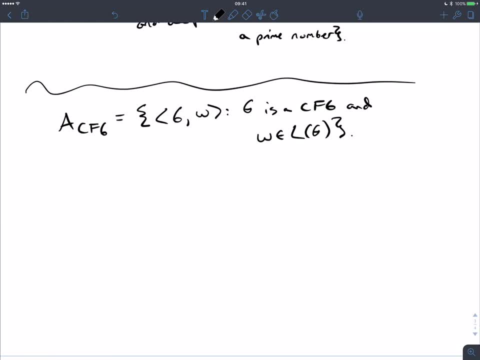 Because CFGs are inherently non-deterministic. I don't know which rule to apply And I don't know if, after a while, I may or may not end up with the string I want right. Is there some easier representation of CFGs that we saw? 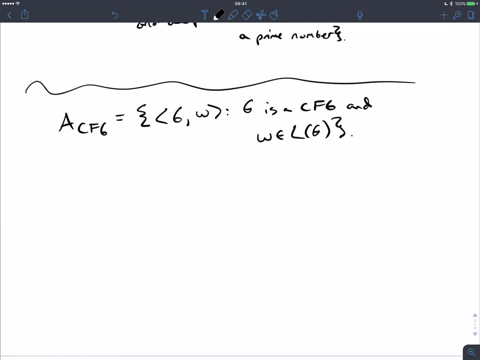 Chomsky normal form. If we have a grammar in Chomsky normal form and an input of length n, do we know how many rules to apply? Yeah, how many? was it? Four, Five? We actually showed a derivation in class. 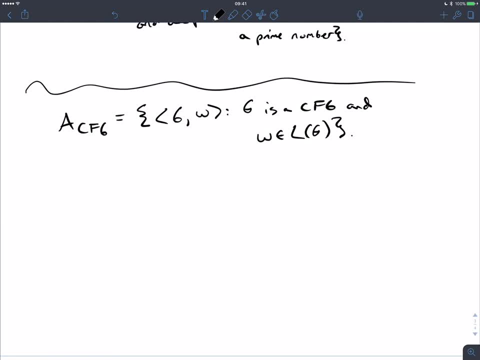 It was 2n minus 1.. Is 2n minus 1, once we get the string finite, Is every derivation of length 2n minus 1 finite, A finite number. It's huge. I didn't say this was fast. 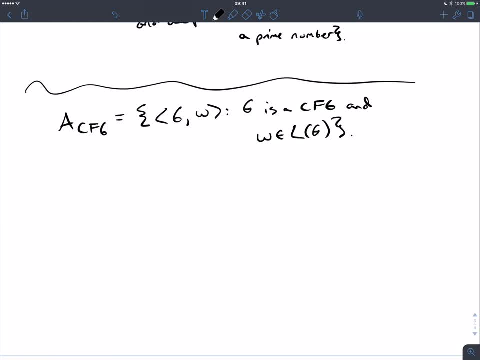 But is it a finite number? Oh, okay, So let's try that. So we're given as input g and w, So I can't say this for any CFG, But if it's in c and f, now I can say something. 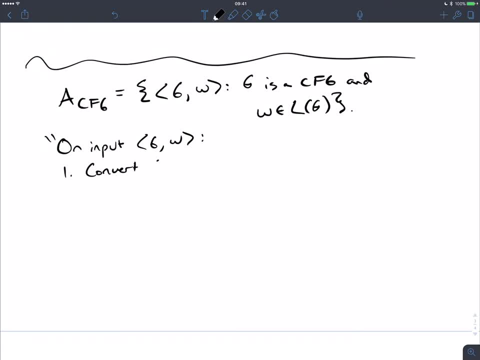 So convert g into an equivalent CFG in. I'm going to call it g prime, g prime In c and f. Does that algorithm take a finite amount of time? The conversion process: Yeah, We were able to show that each of the steps can be done in a finite amount of time. 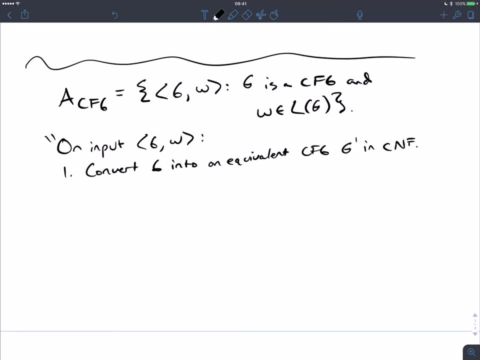 So if it didn't take a finite amount of time, I better not progress beyond step one here, Because then I can't guarantee anything. So there's a little bit of a special case we have to handle here. Do you know what that special case is? 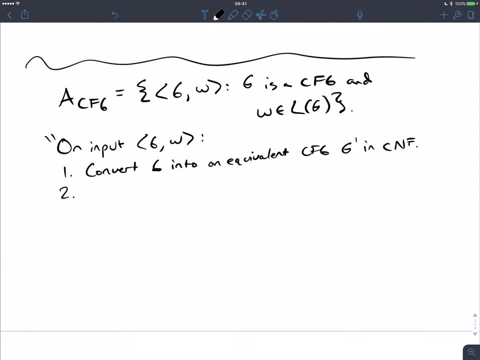 The empty string. What is the length of the empty string? Zero? What is 2 times 0 minus 1? Negative 1.. Can I generate all rule applications of length negative 1?? No, we can't. I consulted with myself. 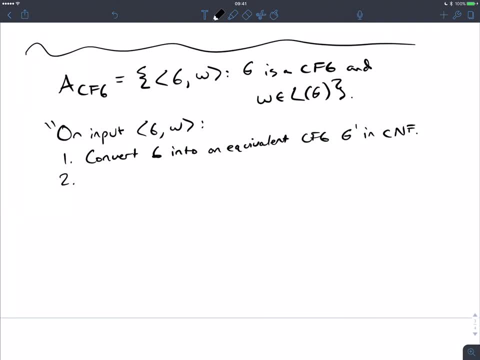 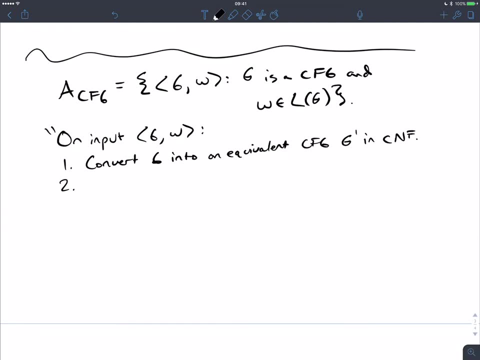 Alright, so we've got to check for the empty string because that's a special case. Is there an easy way I can check whether a grammar in CNF can make the empty string? Yeah, if the start variable makes it, then we're good. 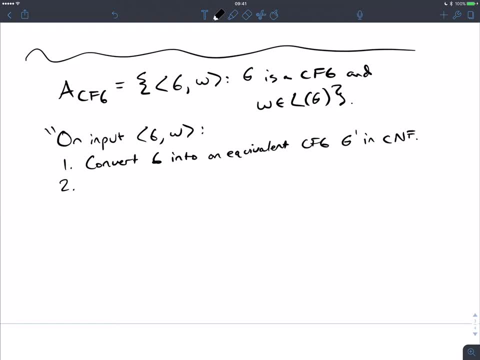 But we've got to check if the input string is actually the empty string, Because there's no reason to do the check otherwise. So if w is empty and s the start variable makes the empty string is a rule, then accept. 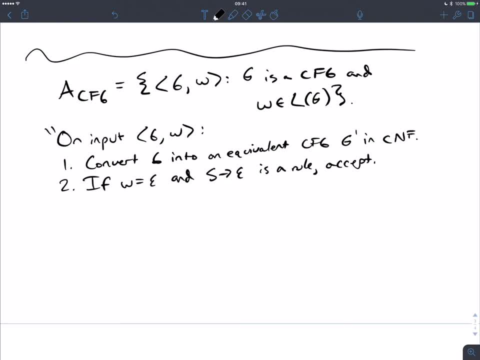 So certainly I can make the empty string this way. Okay, What if s to make the empty string is not a rule I should reject, Because if w is the empty string and there's no rule from the start variable to make the empty string, 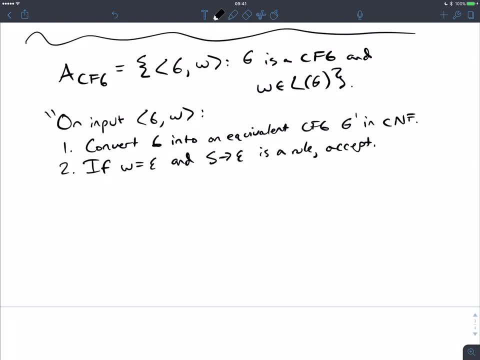 there's no other way to do that, as we have seen. So if w is empty and s to empty is not a rule, we should reject. So if w is empty and s to empty is not a rule, we should reject. 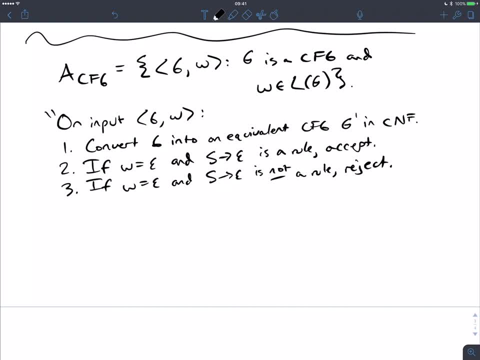 So if w is empty and s to empty is not a rule we should reject. Okay, Yeah, Yeah. Does any grammar in CNF have that first one? No, Only if the original grammar did. No, Only if the original grammar could make the empty string. 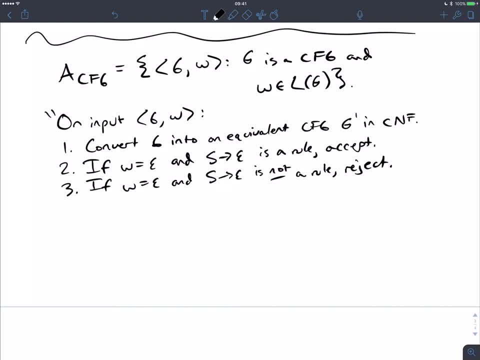 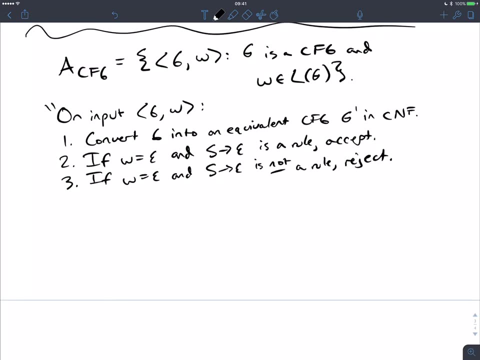 Yeah, because then we propagate the empty string rule up to the top. But if it doesn't make the empty string and we didn't change the language at any point, so it wouldn't have it in the CNF grammar. Okay, So we handled that special case. 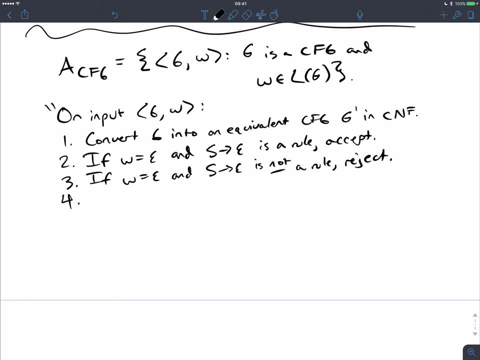 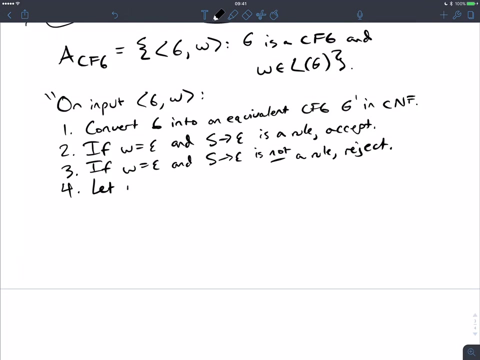 Now what was our idea? to figure out if w can be generated. Yeah, So just check all 2n minus 1 rule applications. Applications of rules of length 2n minus 1.. So let n be the length of w. 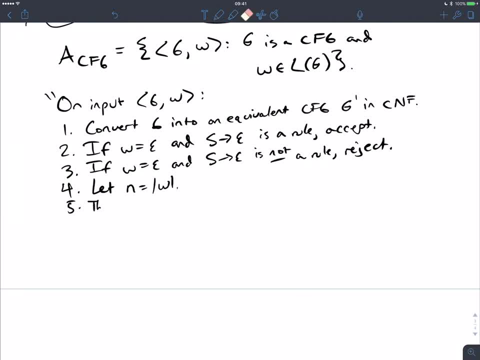 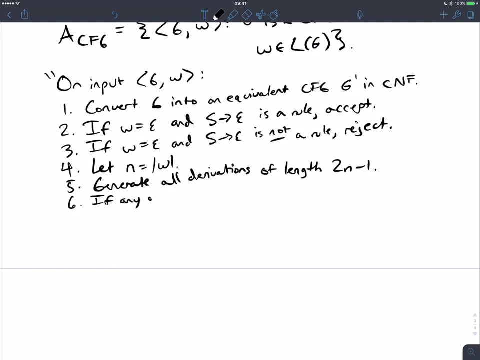 I should generate all derivations of length 2n minus 1.. Okay, Okay, If any of these results in w, accept, otherwise reject. Okay, So a lot of these, since we don't care about how long. 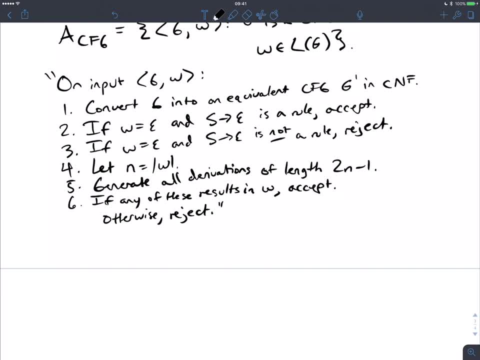 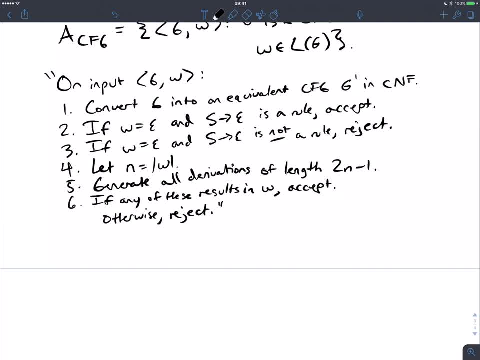 I might as well just try every possibility. There are much faster algorithms. I think chapter 2 mentions one of them, But we're not concerned about that here. Just try every derivation of length 2n minus 1.. And if any of them give w, then we're good. 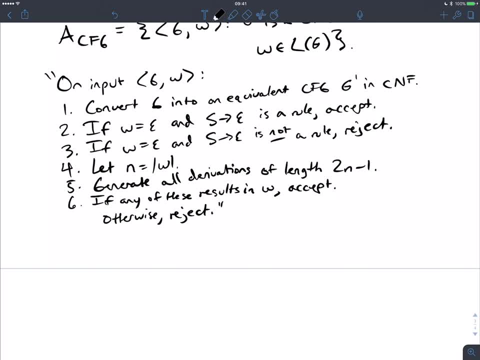 Otherwise we reject. Okay, A lot of these are just brute force, So we're going to do a simulation. Is a PDA decidable? Yeah, Can we convert a PDA to a CFG? Yeah. Does that algorithm take a finite amount of time? 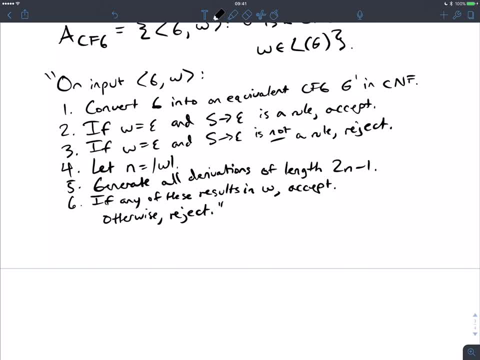 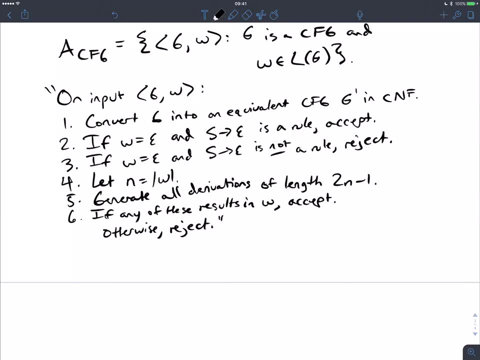 It may take a long time, I don't care. It may take until the heat death of the universe, I don't care, I don't care. So a PDA is decidable as well. If we instead happen to solve a PDA and show it's decidable. 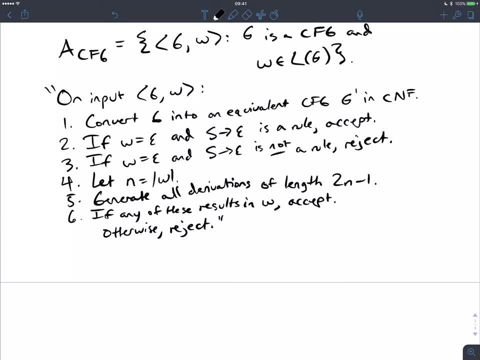 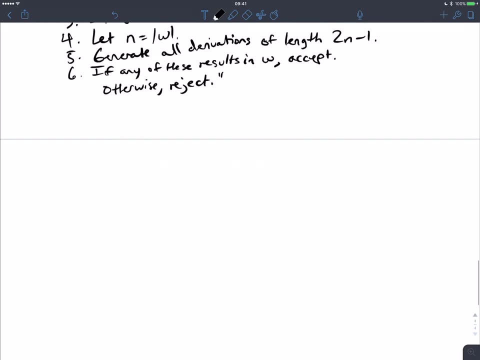 then a CFG is decidable, because we can convert a CFG to a PDA. Okay, Any questions about a CFG or a PDA? Okay, So when we did the regular languages before we talked about the acceptance for each of the models. 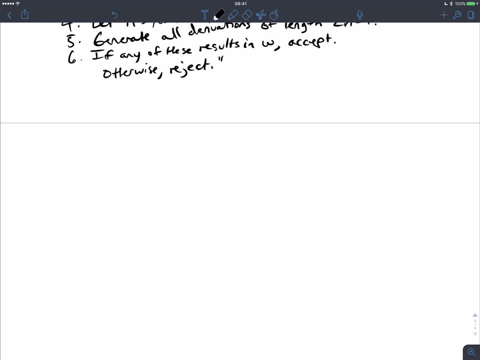 Then we talked about emptiness, So let's talk about emptiness here. So eCFG: So if I happen to solve eCFG, then therefore I also solve ePDA by the same reasoning, So very similar to before. 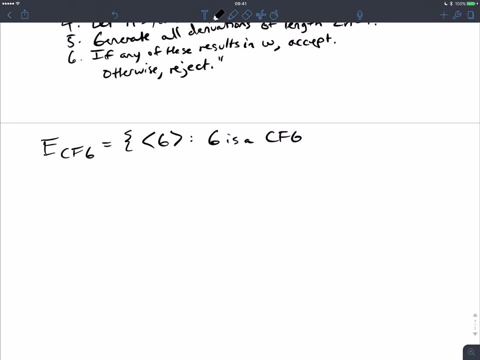 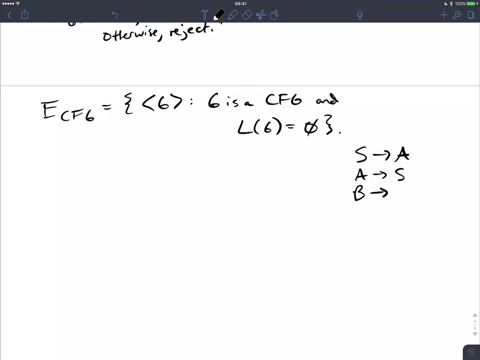 G is a CFG and it generates absolutely no strings whatsoever. So this seems a little bit tricky, because I may have something like this, I may have something like that as a grammar right, where the start variable is S, and since the only rules that I can apply are: S goes to A, A goes to S, and then I can't ever generate anything full of terminals, but there's still a rule that has terminals on the right-hand side. 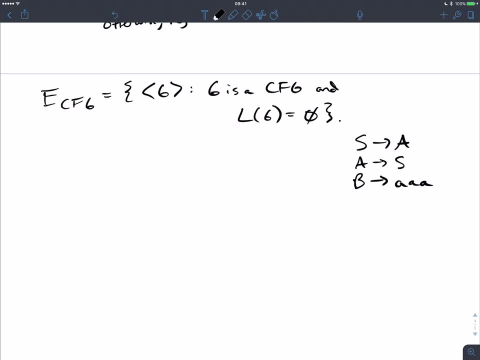 So you could say, well, delete that. But in another grammar I may or may not be able to. For instance, if I have an addition to this, I have something like that: I can never get a string that's entirely full of terminals. 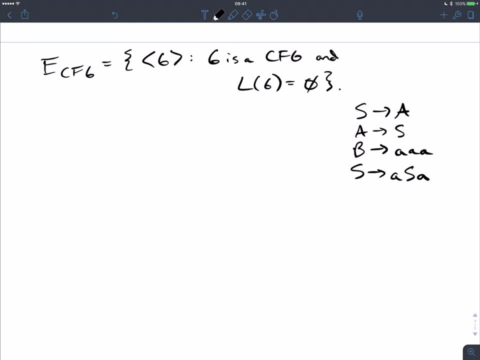 I can get a string of terminals with variables in it just by applying S goes to A, S, A, however many times I like, But I can't get anything full of terminals. So what could I do instead? You could, And that is a strategy. 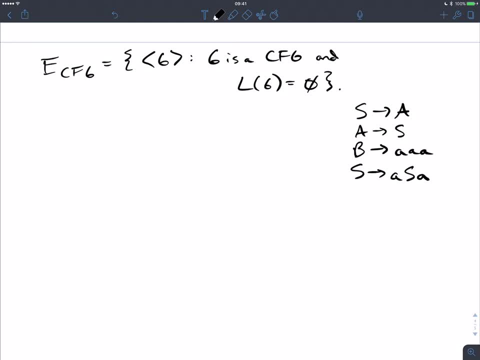 But let's try to think of something other than Chomsky Normal Form. So I'll just give an idea of the Chomsky Normal Form, Convert it to Chomsky Normal Form, Then make a directed graph on the No. that actually won't work because it has two variables on the right-hand side. 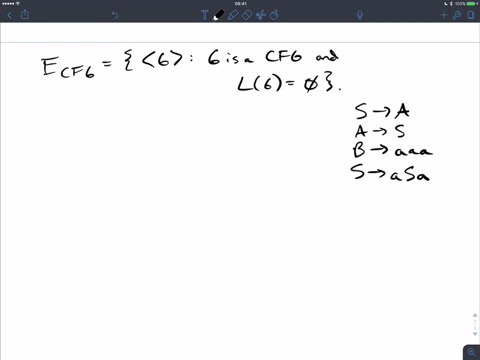 I was thinking that you would have a directed graph: start with the vertex S and you see if there's any path from the start variable to any of the other variables. that happen to make a string only full of terminals. But because there are two variables you can't actually work with that very easily. 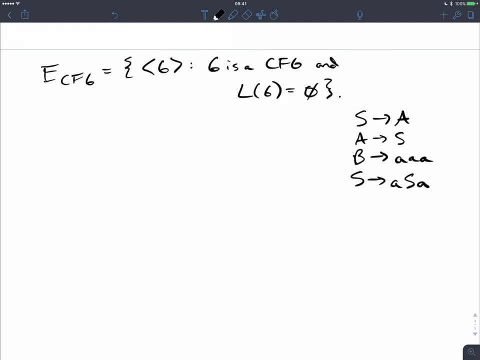 Yeah, you can't work that easily, So what could I do instead? Well, it seems rather enticing. I want to delete that rule, Right, But that rule may or may not be useful, Right? It may happen that the variable on the left-hand side, if I change this, let's say: 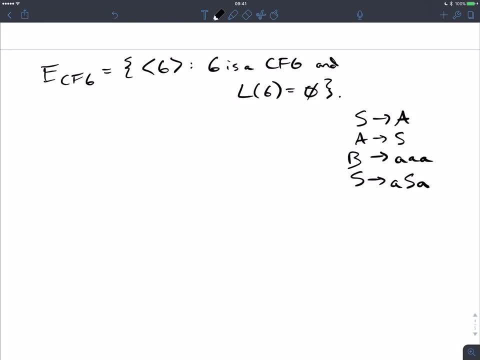 No, I can't change it, But it may or may not be useful for the variable on the left-hand side in some other rule. But maybe what we can do is a bottom-up strategy. We can start with the variables that make terminals. 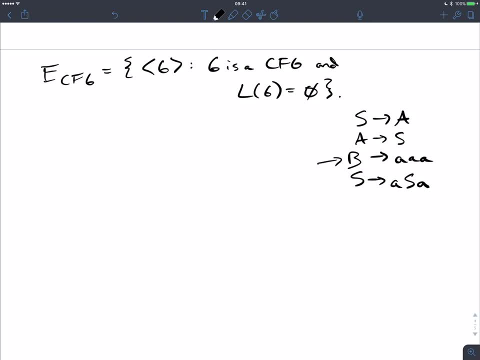 So in this case I know that B, the B variable, can make a string full of terminals, And then I look up and see if I have a rule where all of the variables on the right-hand side can make a string full of terminals. 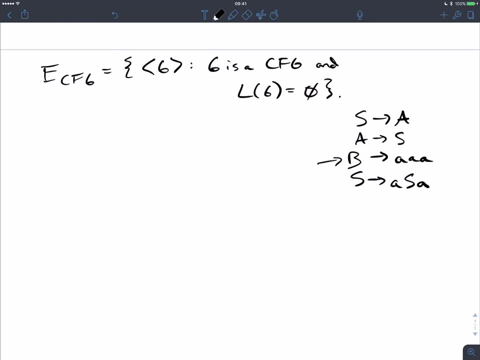 What about Do I know about the variable on the left-hand side? It can make a string full of terminals. Then I just keep going until I check whether the start variable was ever said to make a string full of terminals or not. So that's the idea here. 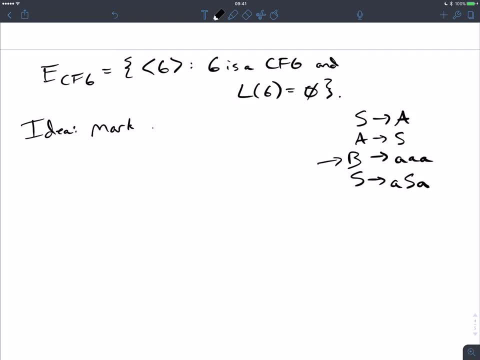 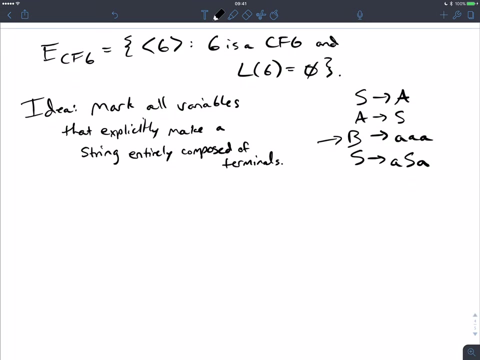 So mark all variables That explicitly make a string entirely composed of terminals. So, like in this grammar's case, I would mark B Right at this step, because it makes a string entirely full of terminals. And then, for every rule, if all variables on the right-hand side are marked, then mark. 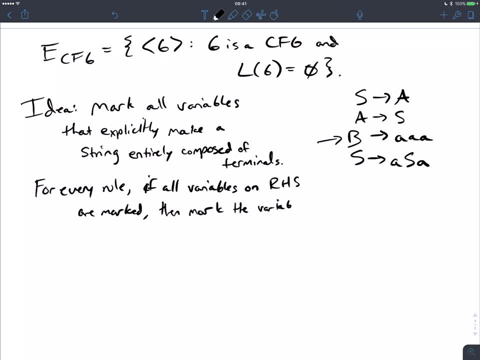 the new variable on the left-hand side, And if, at any stage, I look through every single rule and I don't mark a new variable, then there's no point in me doing this process again, And so therefore, I'm done. 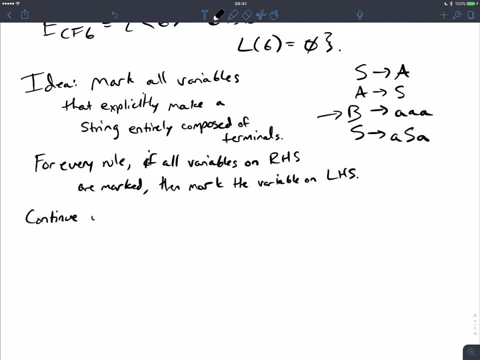 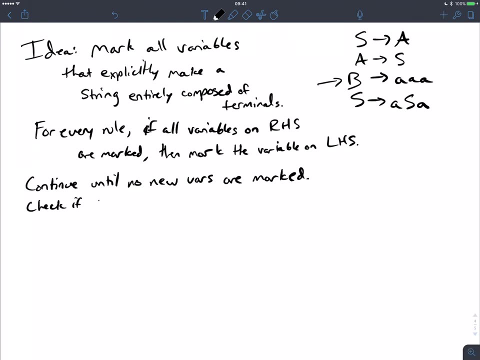 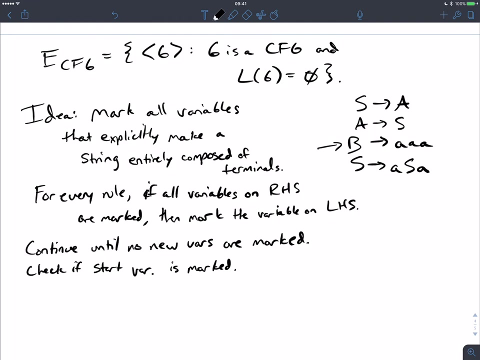 So continue until no new variables are marked. Then check if start variable is marked. Okay, So I just check if the start variable's marked. 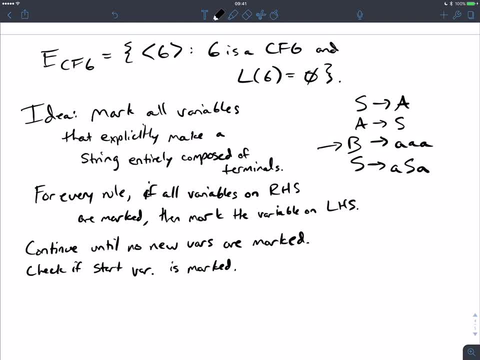 Then there's some other variables for which it was marked, for which they were marked, And then, therefore, there were some other variables maybe that generated a string full of terminals. Okay, So, like in this case, I would mark B. 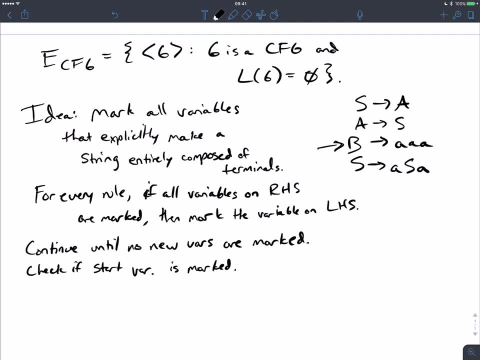 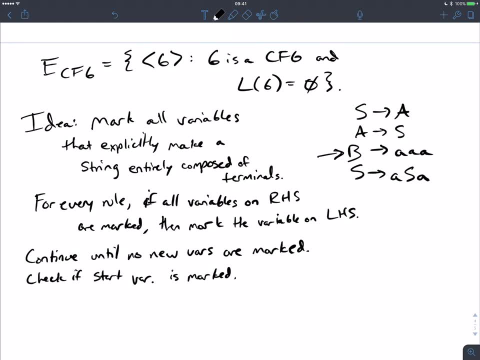 But since B does not appear on the right-hand side of any other rule, then no other variable is marked, And so therefore, since the start variable S was not marked, therefore I can conclude that this grammar's language is empty. 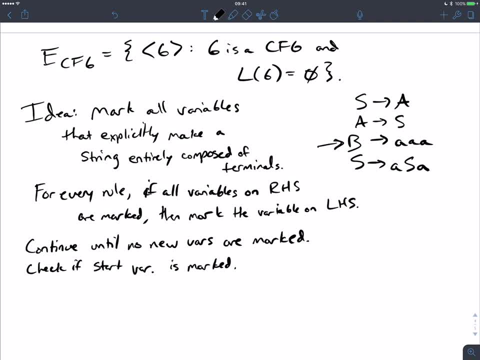 Because there's no way to get to the parts where it actually makes the terminals. Sorry, makes only terminals. Yeah, If the start is marked, we reject. If the start is not marked, we accept. Yes, So, Yeah, So if 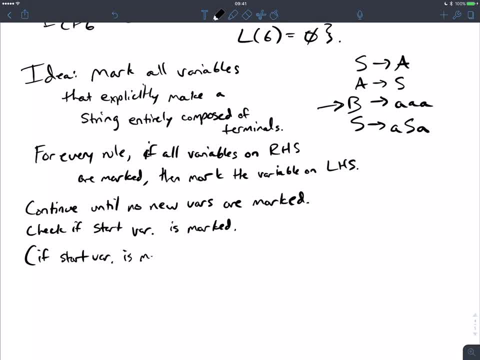 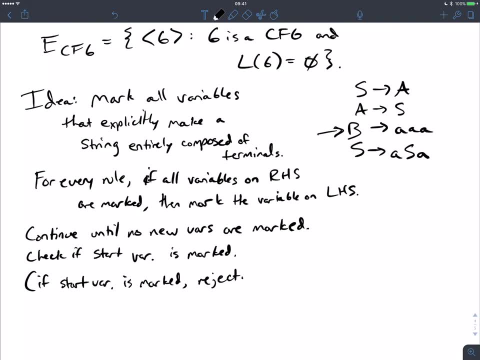 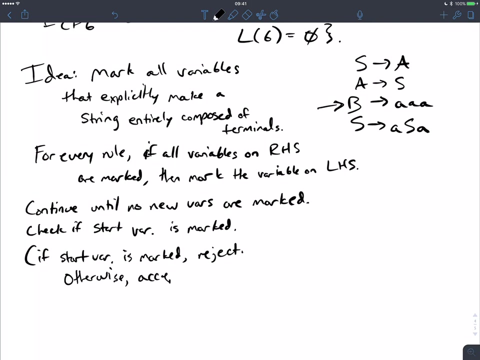 start is marked, in this case we reject. Why do we reject here? Because we just determined that the start variable can make something full of terminals. Then otherwise we accept. So I'm not giving the on input, whatever. 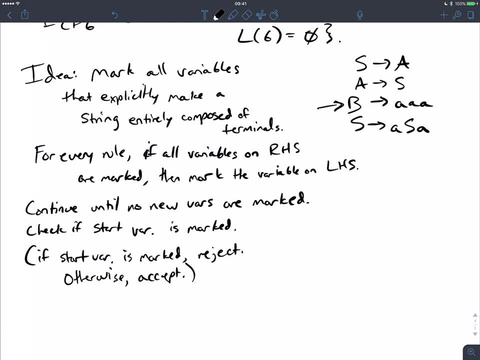 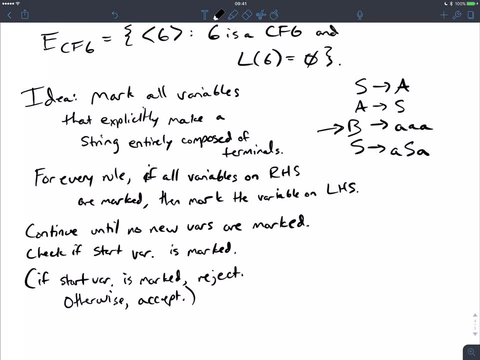 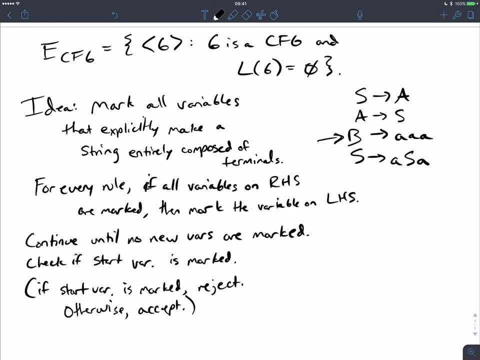 But this is just exactly what you would put in a description like that. Okay, Yeah, Yeah, We should check. Great, Great question. So could I mark all variables? that So the first part where they explicitly make terminals in a finite amount of time. 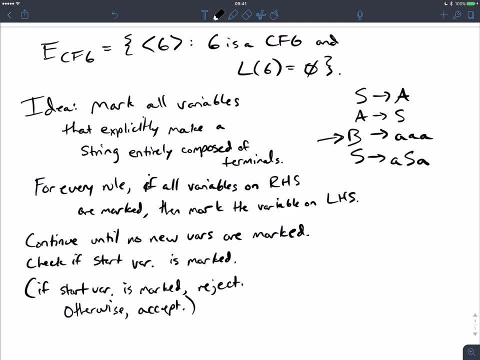 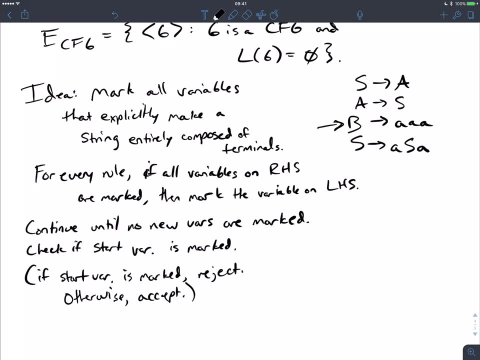 Yeah, There's only a finite number of rules and I can just check on each one Easy. What about this recursive thing Where I keep doing the same process over and over and over? Could that run for an infinite amount of time? No, 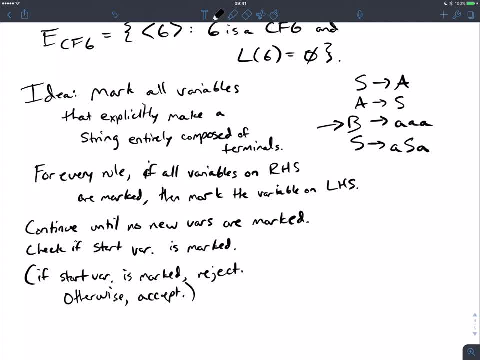 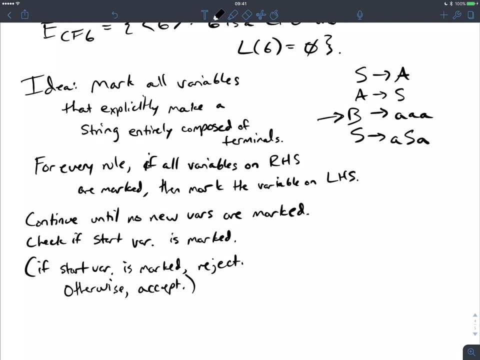 Why? Yeah, If I mark a new variable, then I keep going. But there are only finitely many variables, So this loop can only progress a finite number of times. Okay, And so this keep going until new variables are marked. loop. 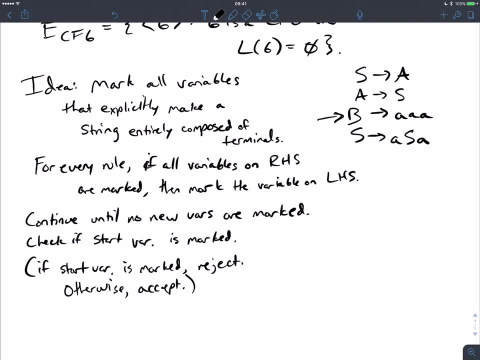 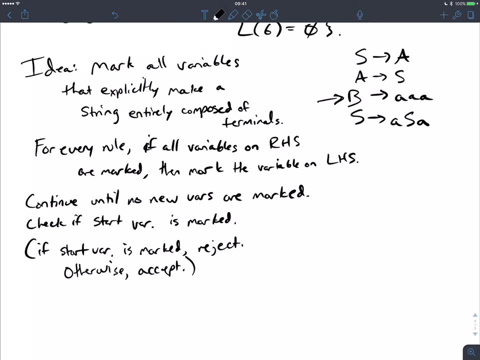 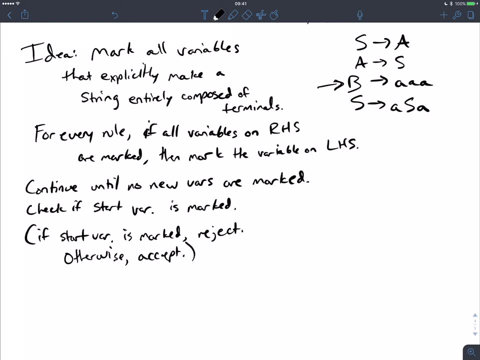 That can only happen a finite amount of time. So therefore that we're good there. Check if the start variable is marked Again finite amount of time, And then rejecting and accepting that's finite as well. Any questions? Yeah, 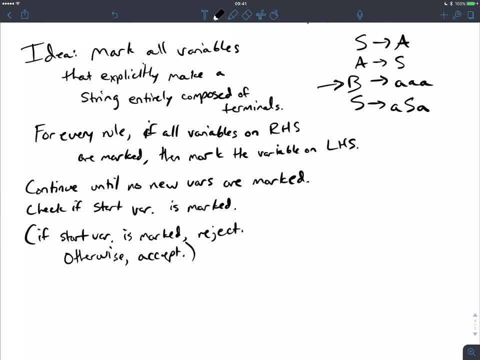 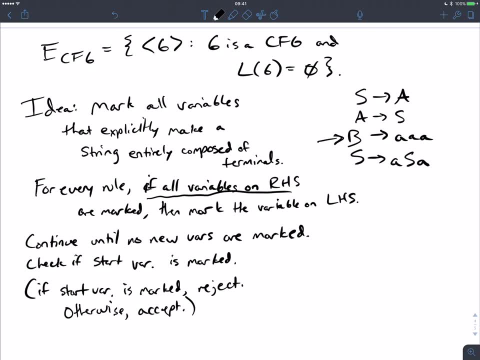 You don't need to have a case if it generates only terminals, Not terminals. Well, I say that here: If all variables on the right-hand side, Yeah, And if it happens that one of them- I've not yet determined that it can make terminals. 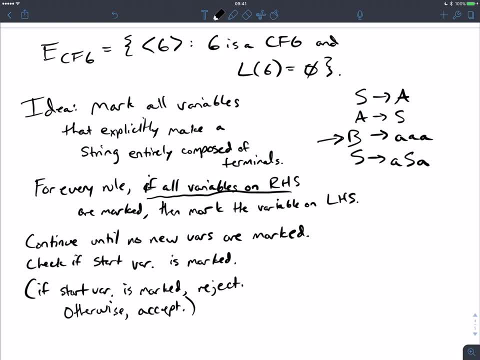 at all, then I can't mark the one on the left-hand side necessarily, But I'm going to go through multiple times and keep going until I can't mark a new variable. Any questions about this? Yeah, I don't know. 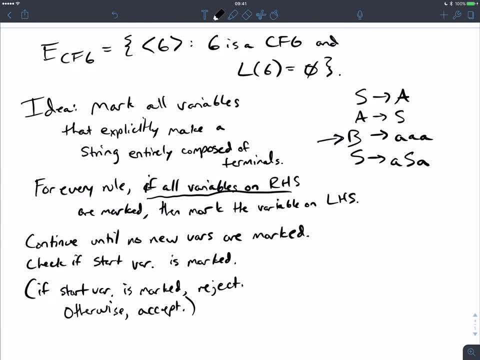 I was going to ask one of these questions, But like, if there's a rule that goes to the law, Or if the state comes to the rule that, like a variable, is the rule that's alternate, and also like 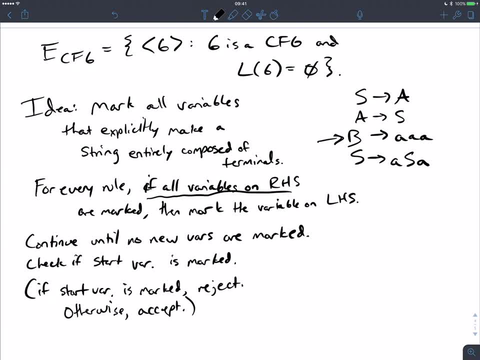 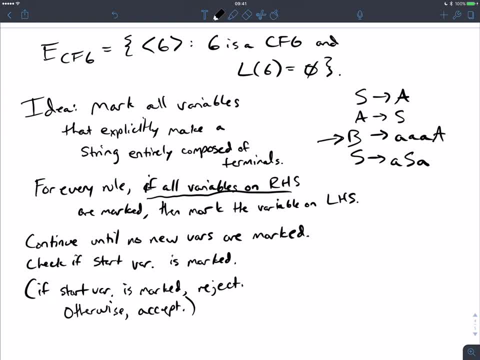 Yeah, Yeah, Yeah, Yeah, Yeah. No, Not necessarily, It doesn't matter here. So you mean multiple variables, like that? That just means multiple rules, Right, But like if there's a mixture of, like all the. 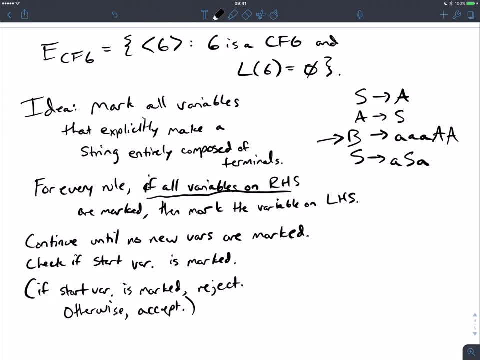 It doesn't matter. I look through every single rule and I mark that single variable in everywhere. I mark the variable, not the rule, Because I can choose which rule to apply. I don't have to pick that particular rule. I can pick any rule with that variable on the website. 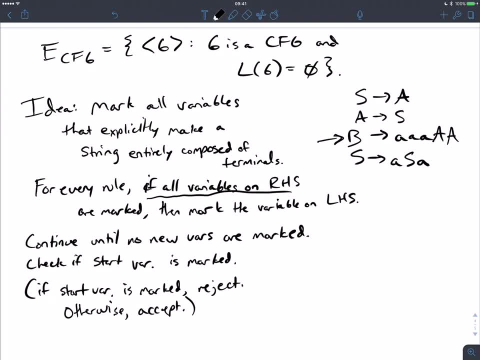 I don't mark terminals, I mark variables. Right now we would no longer mark B. Yeah, I would no longer mark B. I actually wouldn't mark anything because there's no rule with only terminals on the right side. Other questions: 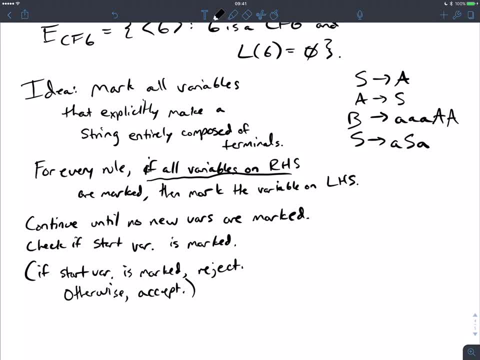 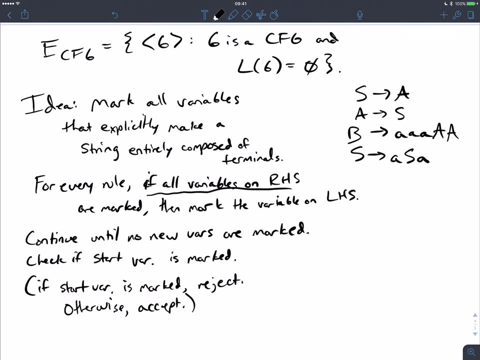 Yeah, no, here, like in this example grammar, I can't mark anything And so therefore, since it's not marked, it can't generate any string of terminals. So what is the language of the grammar? It must be empty because it can't generate any string of terminals. 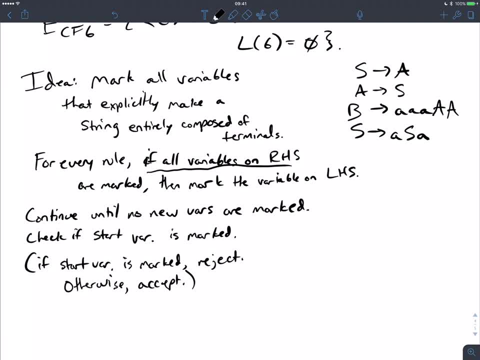 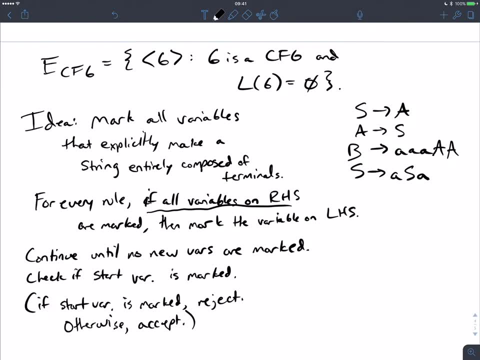 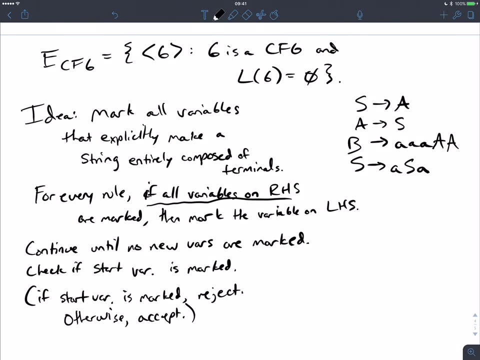 No. so I say here: if the start variable is marked, then we reject Meaning that the grammar has something in its language, Because we're trying to decide emptiness And then otherwise we accept Other questions. So something like this: Right, 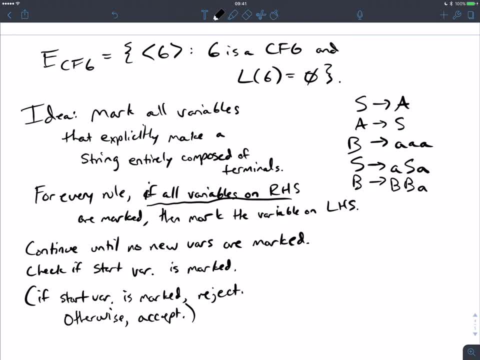 Yeah, Yeah, Yeah, because there is a rule with B on the left side that can make the only terminals. There is a rule, So I would mark B in all places. I'm marking the variable, not the rule, Because I can choose the rule.